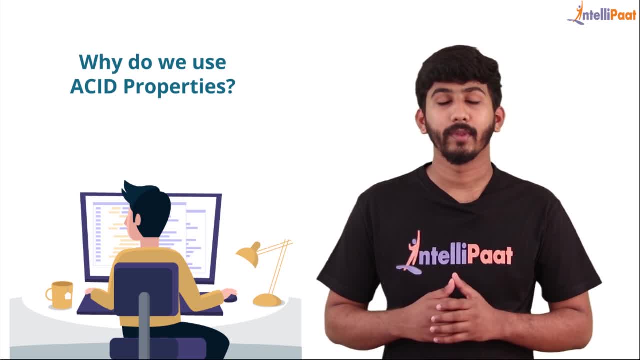 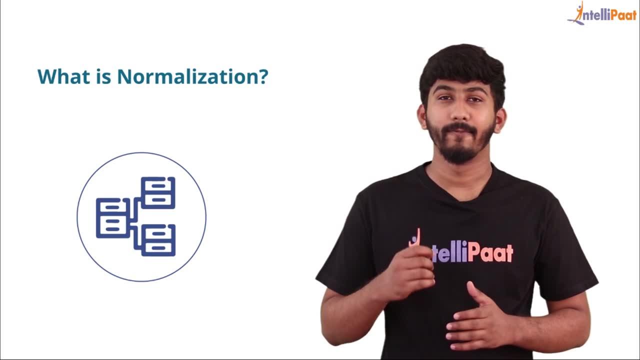 we'll be learning why do we use asset properties, with a quick demo. After that, we'll be learning what are asset properties. After that, we'll learn what is normalization And, finally, we'll be learning what are the types of normalization and how it works. So, guys, 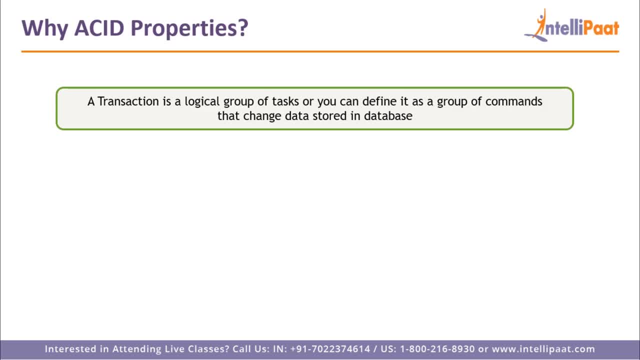 now let us move on with the session. Let me just start off with my first topic, which is why asset properties? All right guys, Now when I talk about asset properties, I'm going to start off with the first topic, which is why asset properties? 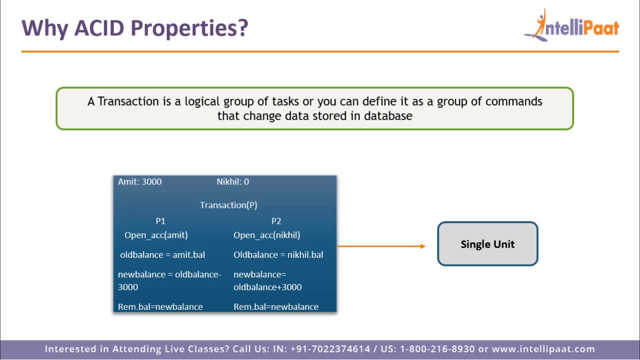 Or when I'm trying to explain you why did asset properties came into picture. So, in order to know that, you guys should know the first and foremost important topic, that is, transaction, So well, a transaction is nothing but a logical group of tasks, or you can define it as a group of. 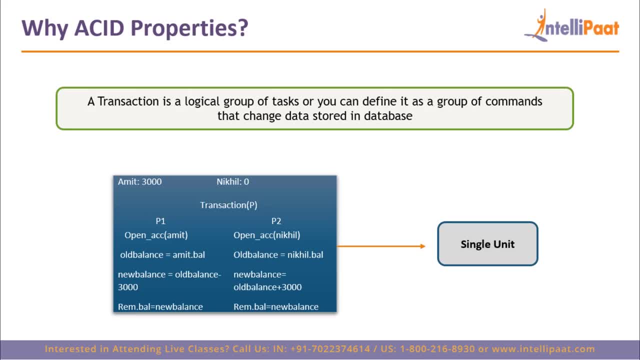 commands that basically change our data, which is stored in a database. A transaction is always a single unit. That is, once you're doing a certain transaction, it is done once and it's like a cycle which has a lifetime, So you have to execute one transaction or you can do one. 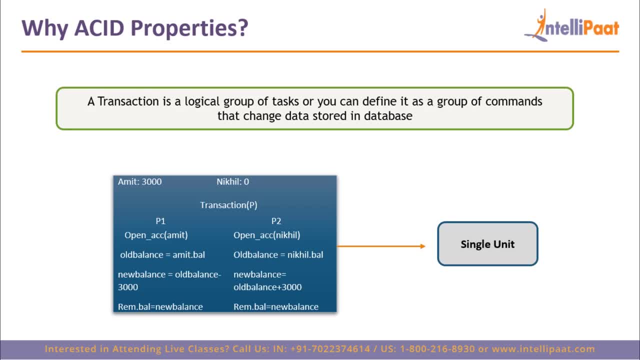 work at a time. In a very simple word, I can say that if you're doing a certain transaction, then you can do one work at a time. Now let me move on and give you a small example related to transaction, so that you guys will get a clear picture of what it is. So let me just minimize. 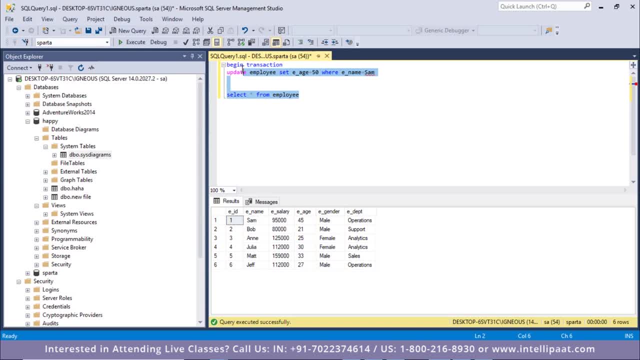 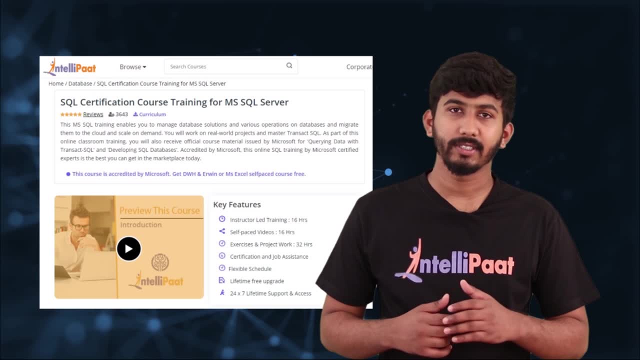 this part and open my SQL Server Studio. Let me just exit this code. Okay, guys, a quick info. If you want to become a certified MS SQL Server professional by Intellipaat, you can check the link in the description. Now let us continue with this session. 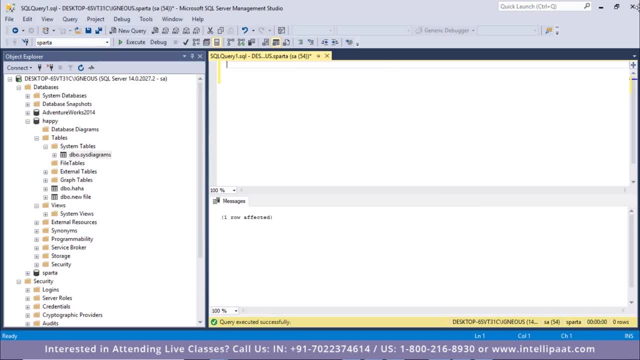 All right. So when I begin my transaction, what I'm going to do here is I'll be writing: begin transaction. Now, under this, I'm going to make use of my SQL query statements. that is update. So update employee, which is my employee table. All right, Set the employee h. that is the abbreviation I'm. 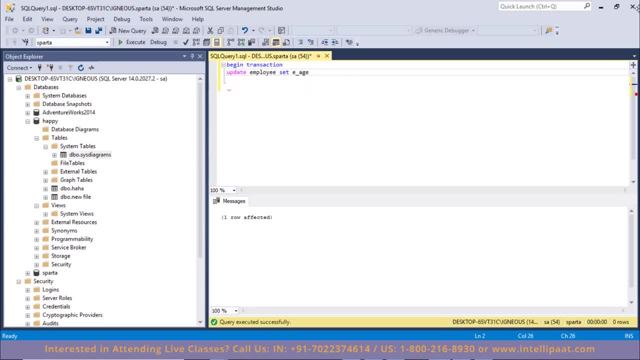 making use of that. yes, e underscore h is equals to- let's say it should be- 50,- sorry, 50, where employee name is equals to Sam. All right Now let me just select these two statements, what i have written here, and execute it so, as you can see, it shows one row has been affected. 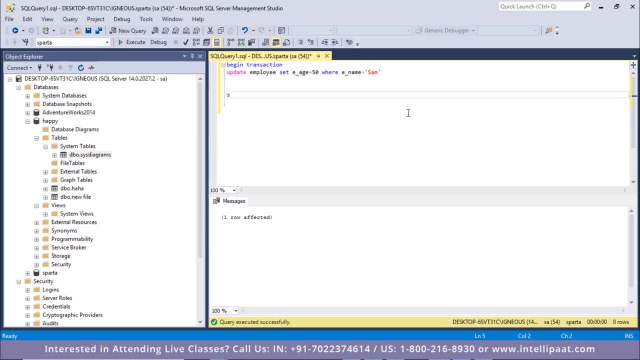 now, in order to fetch my results, i'm going to simply make use of the sql statement, that is, select star from employee and execute this. so now, guys, as you can see, our previous age was, or the previous employee age for the name sam, was 45, and now it has been updated to 50.. now a transaction is not complete. 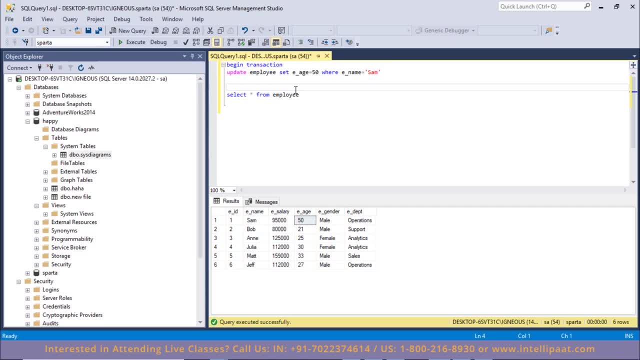 without the two operations that are, rollback and comment. now let's say i want to roll back this operation, that is, whatever employee age which has been modified or the new employee age. i want the previous employee age back. so what i got to do is i'll just go back and simply type here: rollback. 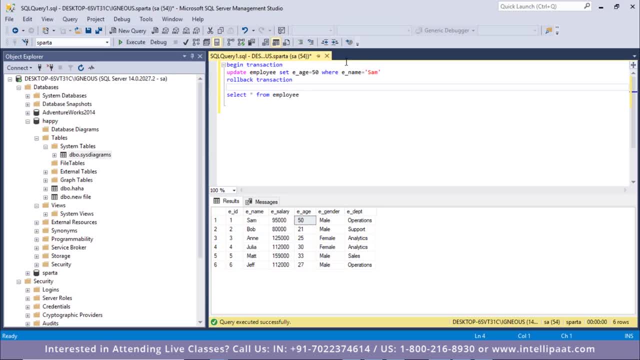 transaction. all right, just give this space over here and select this so it shows commands completed successfully. now i'll move on and select this part and execute it again. so, as you can see, guys, our previous employee age has been rolled back. so rollback is one of the sql statements with which basically rolls back your. 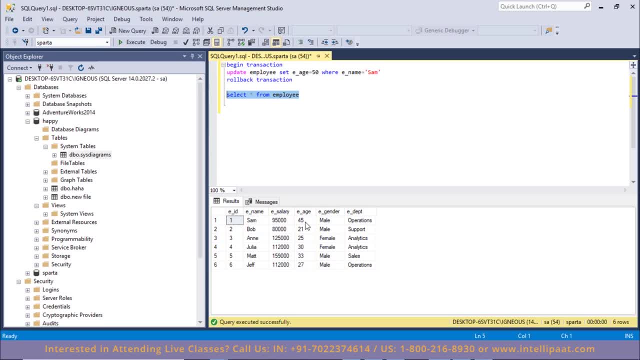 entire operation. now the main reason why i'm explaining you these two parts. i'll i'll tell you the reason later. let me just show you how do you commit a certain transaction. now, let's say, i want to remove this rollback transaction statement, so i'll just delete this part and i'll again select these two statements. 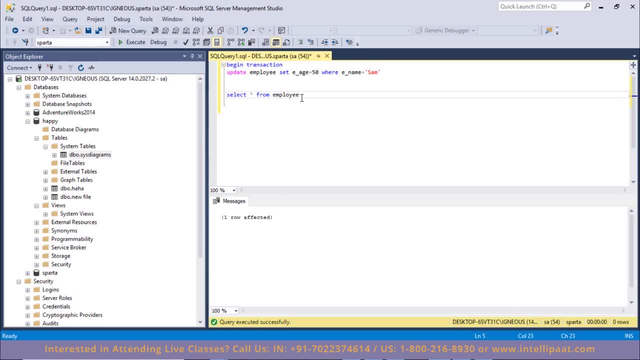 execute it and it shows one row has been affected. now i'm just going to select my select star from employee statement and now i'll execute it. so now my employee age has been modified to 50.. now let's say i want to commit this particular transaction, so my commit statement will commit. 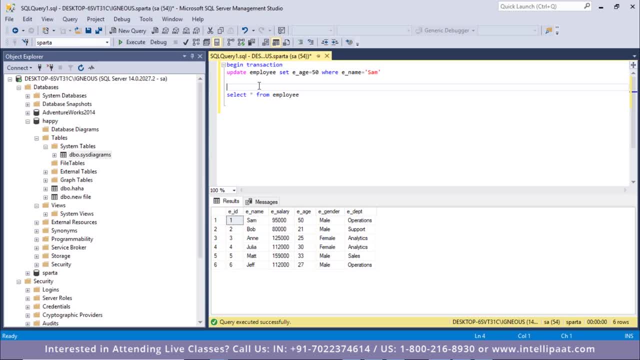 the whole changes or the whole transaction. so i'm going to commit the whole changes or the whole modification, what i have done in the db forever. so i'm going to write or make use of commit transaction. all right, let me just give space over here and select this part and execute it all right so it shows the message. commands completed. 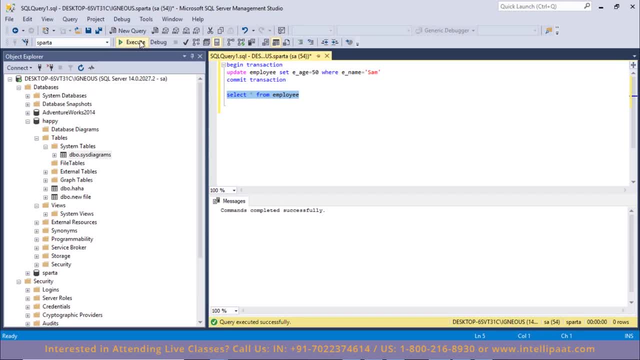 successfully. now i'm going to simply select this statement, that is, select star from employee, and execute this part. all right, so now our transaction has been committed. okay, guys, a quick info. if you want to become a certified mssql server professional by intellipaat, you can check. 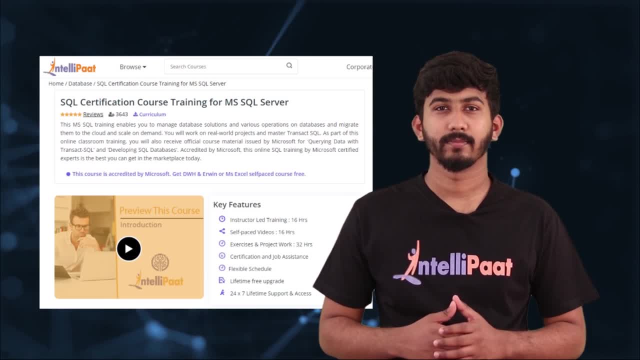 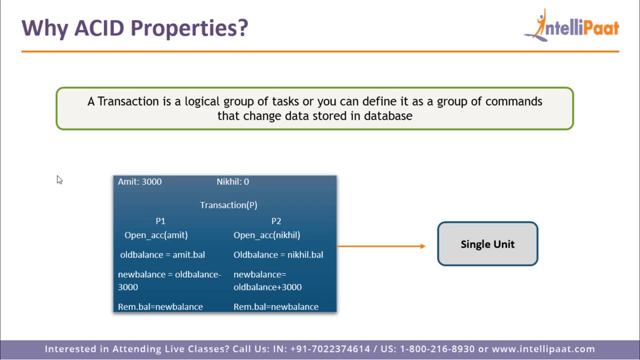 the link in the description. now let us continue with this session. i just gave you a hands-on session of transaction, where i was beginning a transaction and i had taken into account of an employee table where my first process was i was basically updating the employee age from. 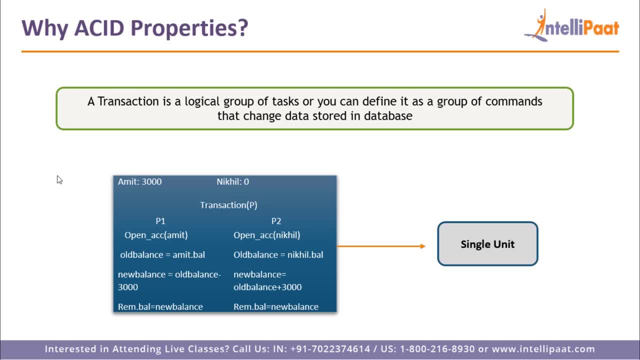 a certain number to a different number, After which I tried making use of the SQL statement that is rollback. So, using that particular statement, I was able to get back the previous agent of the employee, which was existing in the employee table, And then I made use of the commit transaction, due to which the modification or the changes 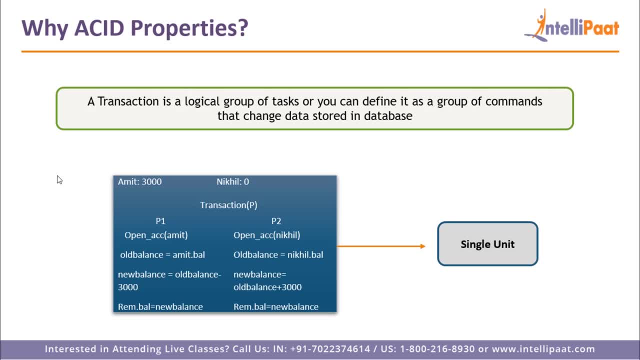 what I had done in the database will always get committed or will always be saved forever, Like even if the system crashes, it will be there existing on our DB. Now let me just move forward and talk about the various aspects. why did asset properties? 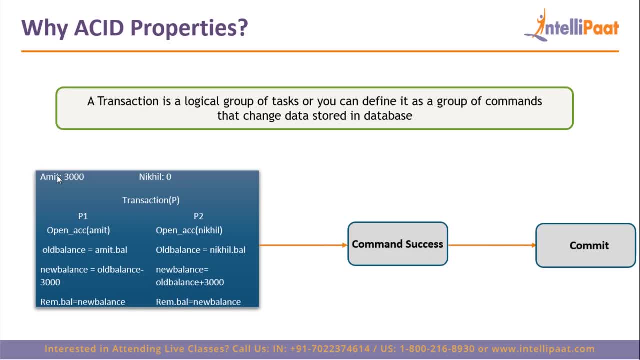 came into picture. Now let me take a use case where we have two people. So one guy's name is Amit and the other guy's name is Nikhil. Amit's bank account has 3000 rupees and Nikhil's bank account presently has zero rupees. 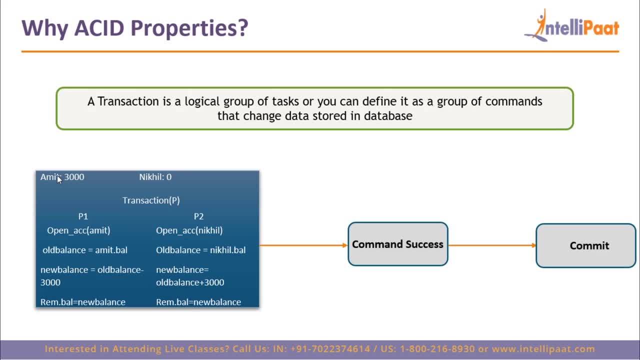 So what I'm trying to do is I'm trying to transfer this 3000 rupees from Amit's bank account to Nikhil's bank account, So when the transaction P comes into picture. So I have divided it Into two parts, that is, P1 for Amit and P2 for Nikhil. 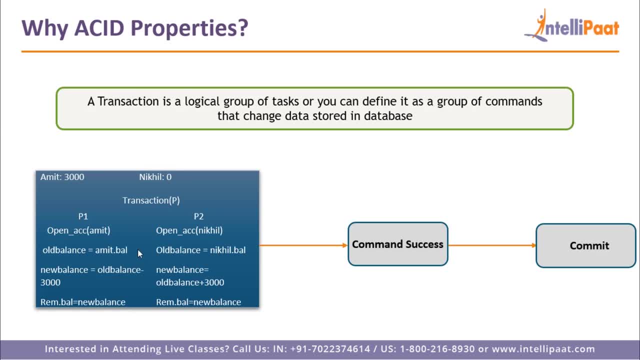 Now I've written a small pseudo code over here which basically talks about that. I'm opening Amit's account and initially Amit's balance is equals to the new balance. Now, when my deduction of money will take place, then that 3000 rupees will get deducted. 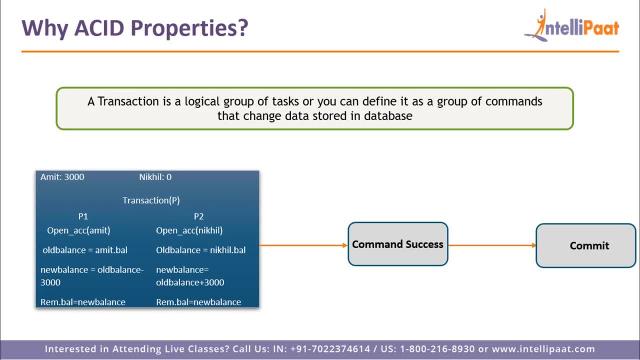 and then my remaining balance, or my new balance, will be equals to the remaining balance. that will be equal to zero. Moving forward to Nikhil's bank account, I have written the same algorithm, But here Zero will be added with the new money that has been credited to his account. 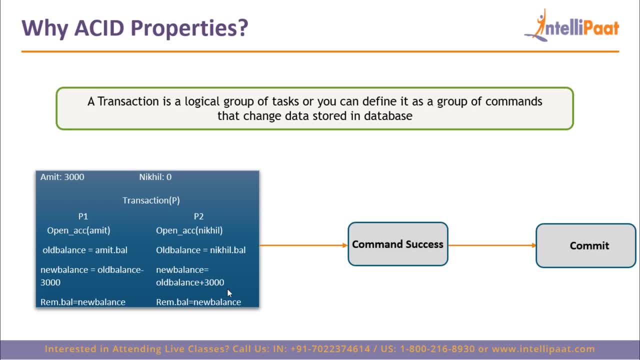 That is 3000 rupees, and his new balance will again be equal to the remaining balance. So now his remaining balance is 3000 rupees. So, guys, this basically forms a part of one transaction, And if this whole operation is successful, then only we can commit the database. Otherwise there can be such cases where 3000 rupees has been deducted from Amit's bank account, but that rupees or that amount Of money never reached Nikhil's account. So in such cases it is basically called as a fraudulent transaction. 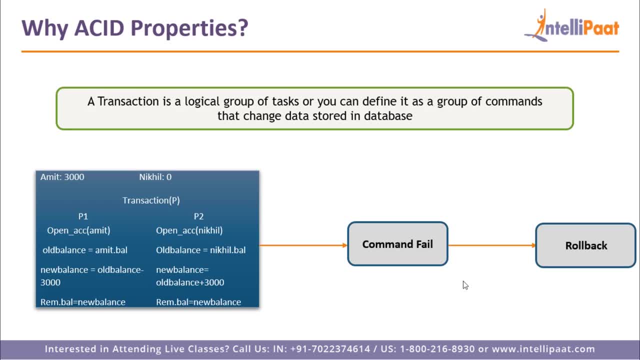 And in such operations are not considered as legitimate when we talk about transactions or when we talk about the reason behind the existence of asset properties, because that transaction or that DB has to go through those principles. And if your operation is failing, then you have to make use of the rollback statement so that you again start. 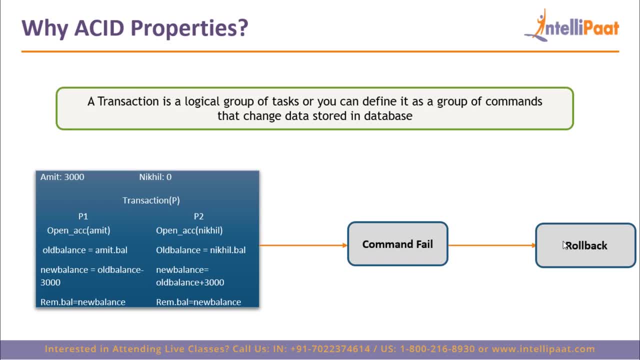 the transaction from the beginning. That's the reason why there are certain guidelines and these properties the DB has to adhere to, And that's the reason why asset properties came into picture. Now let me just move on and talk about what are asset properties. 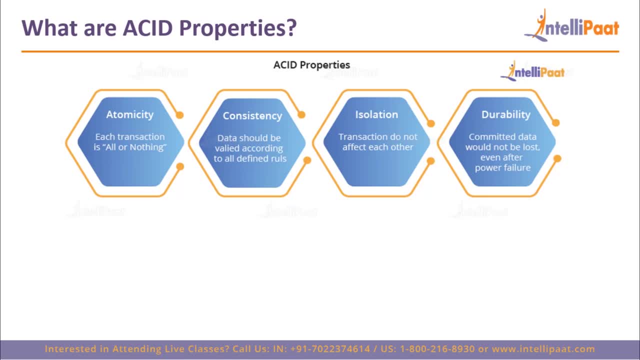 Well, let me just start off by giving you the brief abbreviation of asset properties. So asset properties, basically, are essentially stands for atomicity, consistency, isolation and durability. As you can already see, it is given in the slide. Well, asset properties are again one of the most important aspects of database and I have already given you. 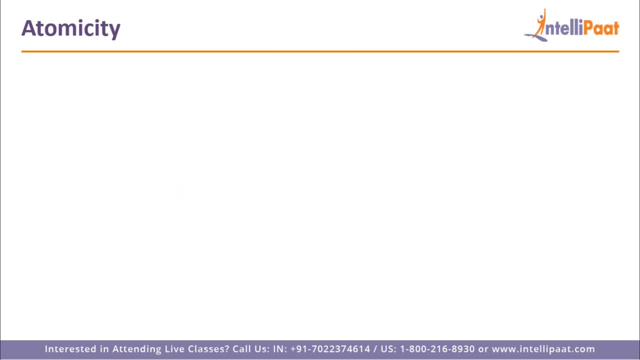 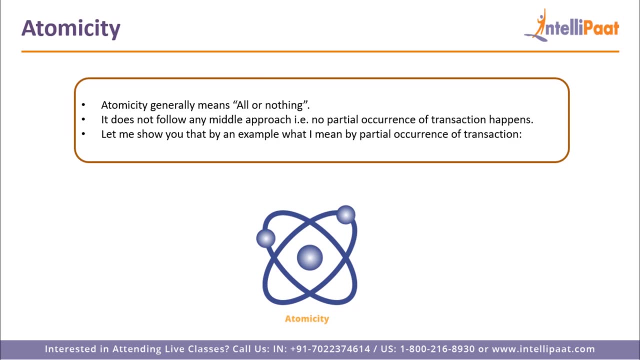 the abbreviation. So let me just move on and talk about what is atomicity. So atomicity generally means all or nothing. Well, again, whatever is written in my slide, it basically says that it does not follow any middle approach, That is, there should be no partial occurrence of transaction happening. 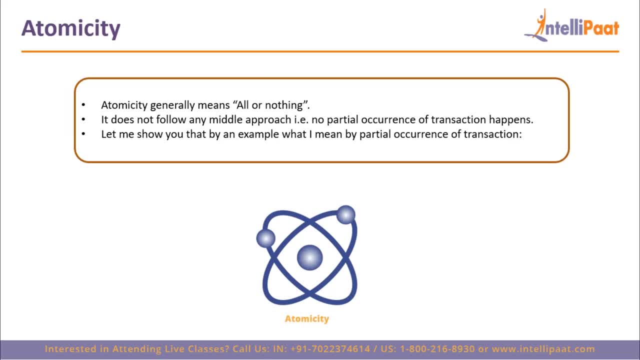 I'm going to be showing you an example of what I mean by the partial occurrence of transaction. So well, what I mean by this particular statement- that is my first statement, which talks about atomicity- generally means all or nothing- is if a transaction is taking place. 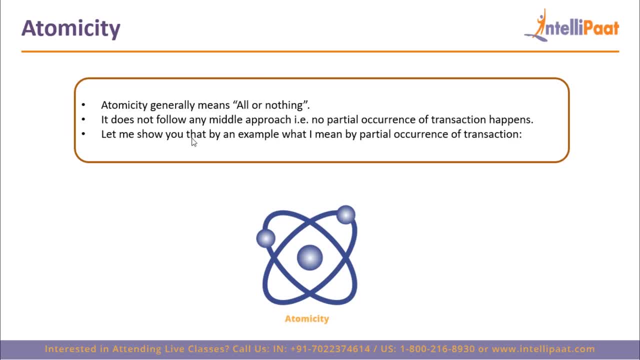 I'll go back to my previous slides where I had explained transaction. So let me just brush in that part up again. So if a transaction is taking place, it has to take place full, Otherwise it will again start from scratch. That is, the rollback operation will be happening and then it will get committed. if that part doesn't happen, 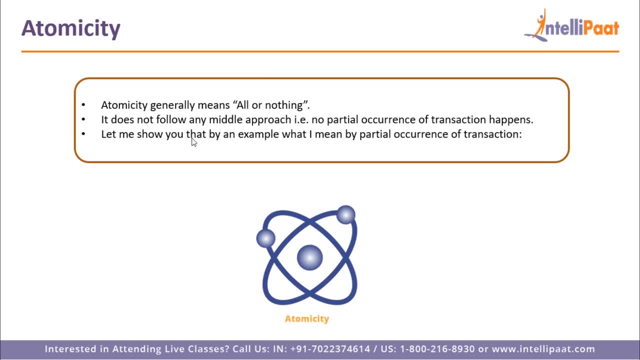 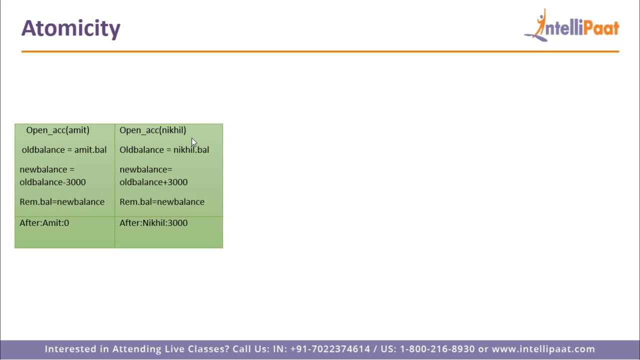 Then Our database will be considered as inconsistent or incompetent, or it will also be called as not a good DB. So let me move ahead and give you the example of those two bank accounts again. So what we did was I have written the same pseudocode. 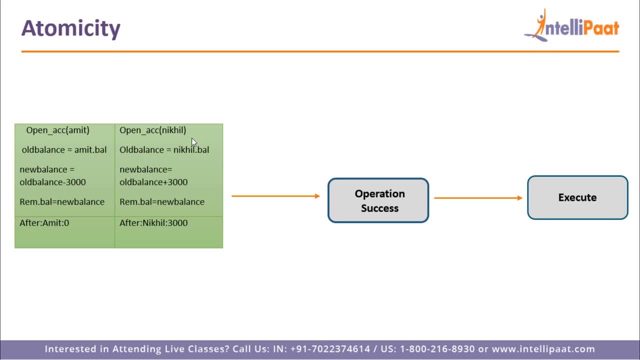 Now what's happening is again. I have taken into picture of Amit's bank account and the pseudocode is talking about deducting 3000 rupees from Amit's account initially, and then that 3000 rupees Is then added to Nikhil's account. 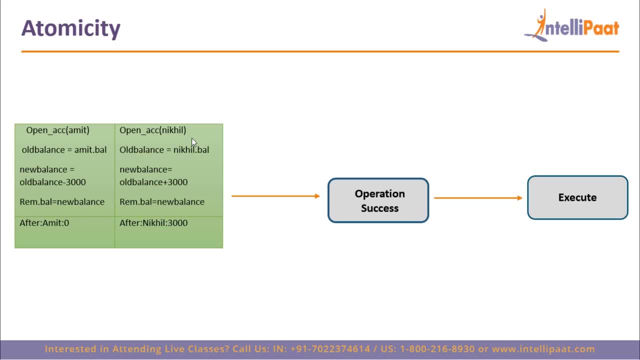 Now this whole part or this whole one operation is called as a transaction. So the operation is success, then you will be able to execute it or you can commit the database. But what if? again, I'll be repeating the same set of statements that if the operation fails in the middle. that is, let's say that the money has been deducted, that is, 3000 rupees is deducted, but that 3000 rupees is not added to Nikhil's account. 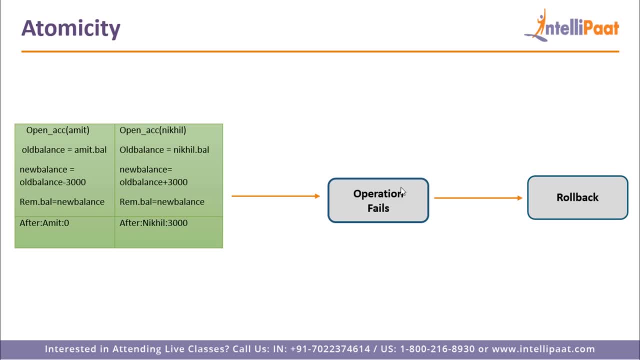 So when this operation is failing, then our operation fails, Then our operation fails, The operation has to again start from scratch, that is, it will roll back and it will start from scratch, where we'll deduct the money from Amit's account and then that money will be added to Nikhil's account. 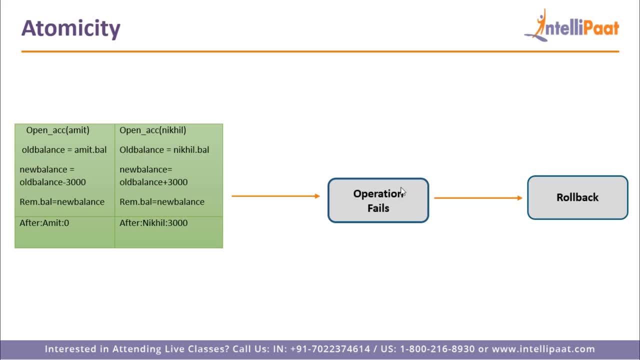 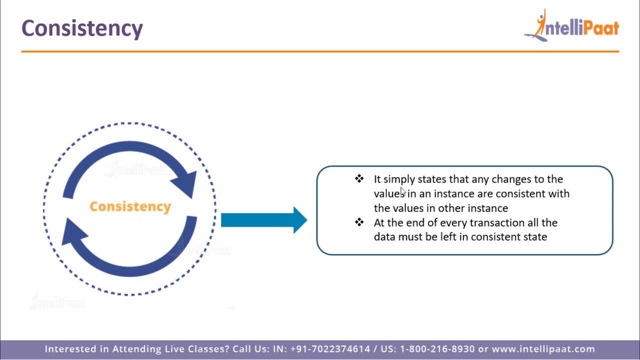 And this is essentially what atomicity means, which is, either it is all or it is nothing. So, moving on to our next topic, which is consistency. Well, consistency is nothing, but it ensures that whenever a transaction has ended. So let's see. 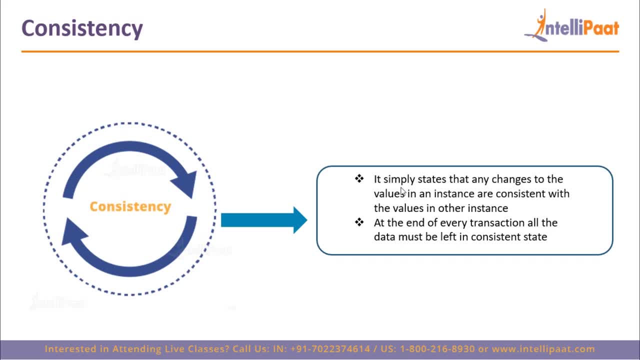 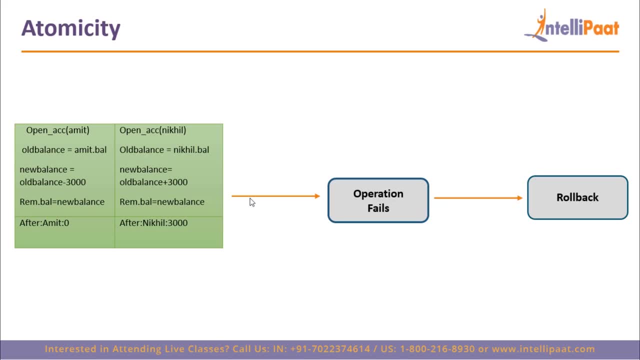 We had deducted money from Amit's account initially and that money was added to Nikhil's account. So let me just go back to my previous slide. I will explain you consistency from here itself So well, when we deducted money from Amit's account and then it got added to Nikhil's account. 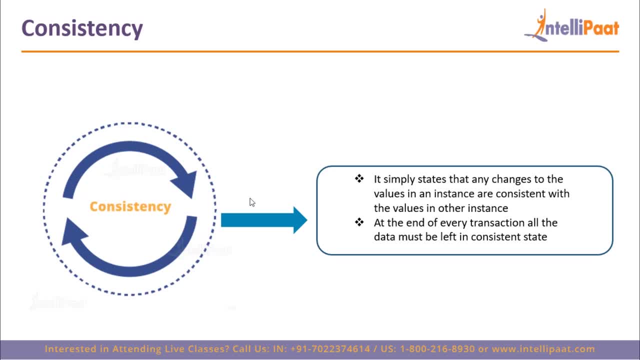 So what happens is the state before the transaction- that is, before Amit's account had 3000 rupees and Nikhil's account has zero rupees- and state of the DB after the transaction has taken place. So the consistency of all the transactions that has taken place has to be the same, which also means that at the end of every transaction, all the data which is left must be in a consistent state. 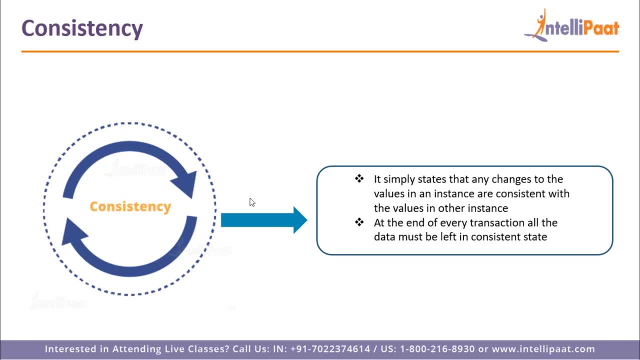 So it has to be 3000 rupees before and 3000 rupees after, And that's how you check the consistency of the DB. or in simple words I can also say it states that any changes which are happening with respect to the values in an instance are consistent. 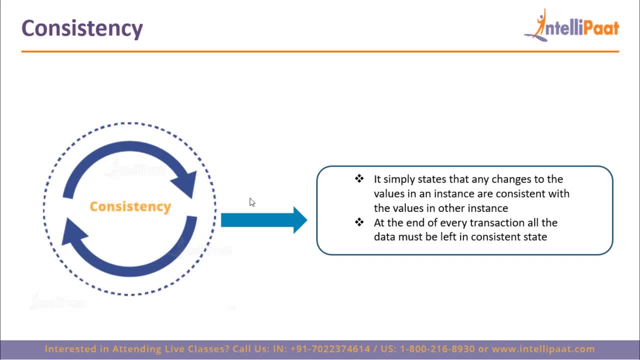 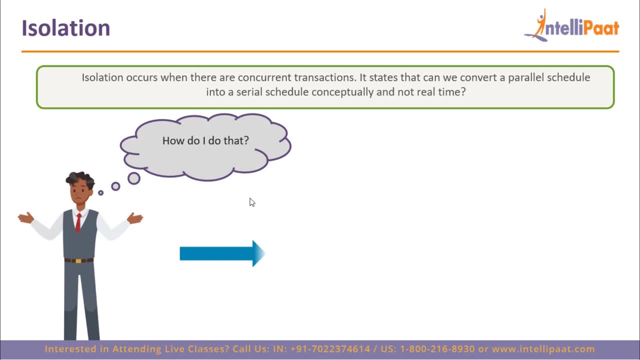 Then it should be consistent with the values in other instance too. Now I'll move on and talk about my next property, which is isolation. Well, isolation generally occurs when there are concurrent transactions, means there are multiple transactions which are taking place. It also states that we can convert a parallel schedule. 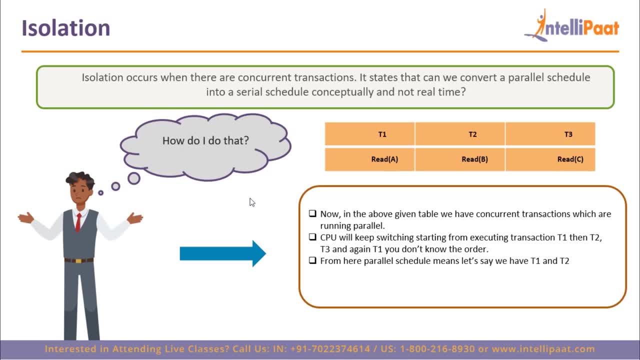 into a serial schedule conceptually and not in real time. Now, of course, you guys must be having a problem in understanding what does this whole statement mean and how do I do that or how do I achieve it In order to understand this. so let me assume a table. So I have written a table over. 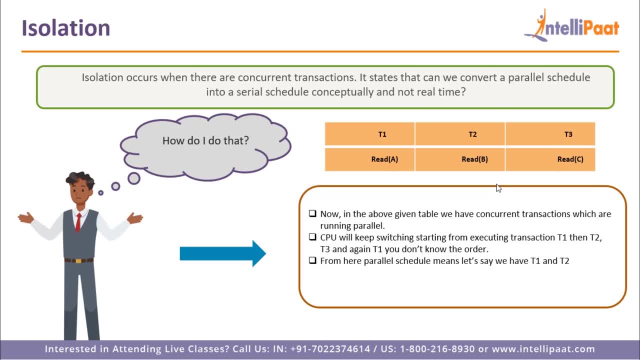 here Now, in this above given table, we have concurrent transactions which are running in parallel. So what's happening is when these transactions are taking place. so let's say we have T1, T2 and T3, and in T1 we have a read statement that is reading A. in T2 we have a. 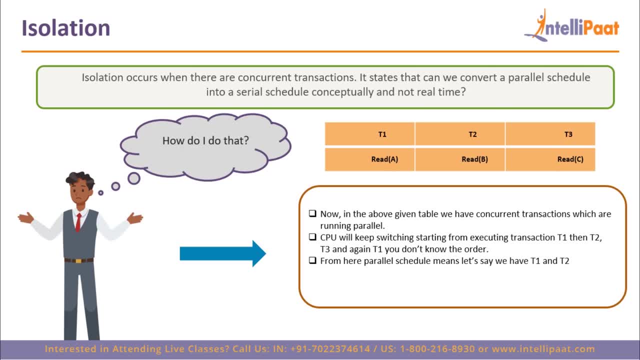 data statement, reading b, and in t3 we have a read statement that is reading c, and all these transactions are running parallelly, or i can say are running concurrently. so the cpu, what it will do, is it will keep switching, starting from executing our first transaction. then it will execute t2, then 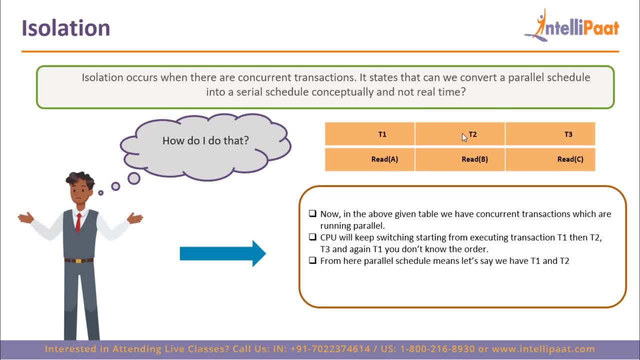 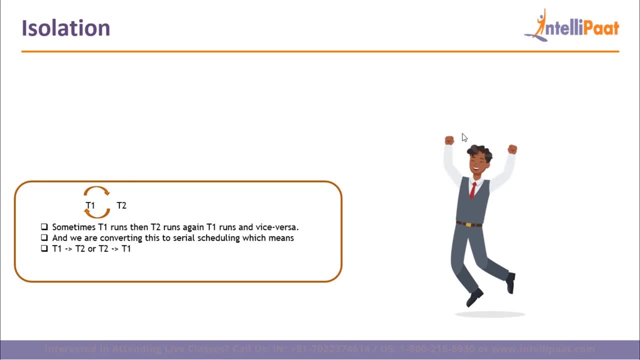 it will go to t3 again, it will come back to t1. so when i say parallel scheduling, what i mean is: so let's say we have t1, okay. so sometimes, sorry so, sometimes, t1 runs and then t2 runs again, it comes back to t1, and vice versa. so none of the transaction is taking place properly, that is, or? 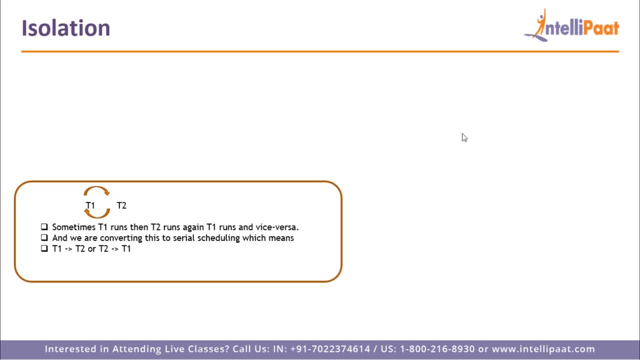 i can say, according to isolation, one process is taking place or one transaction is happening, then subsequently it again switches to the second transaction and it is not getting completed properly. what i'm going to do is that we have to convert this to serial scheduling, which essentially means let the first transaction complete and 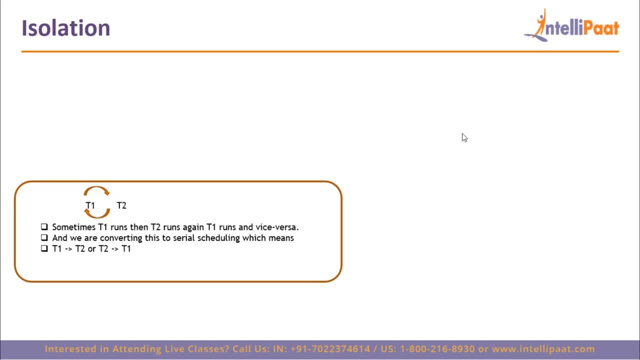 then the cpu will switch to the second transaction. or let the second transaction complete, then the cpu will switch to the first transaction. or let the first transaction complete, then the cpu will switch to the third transaction, or let the third transaction complete, then the cpu will switch to. 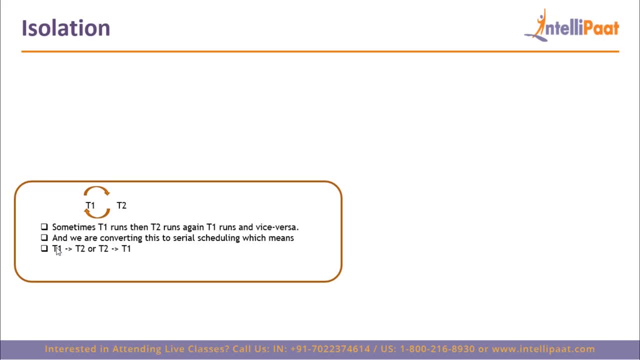 the second transaction which i have shown here. that is, once t1 gets completed, then it goes to t2, or once t1 gets completed, then it goes to t2, or once t1 gets completed, then it goes to t2, or once t2 gets completed, then it goes to t1. now i think this guy is pretty happy after this. 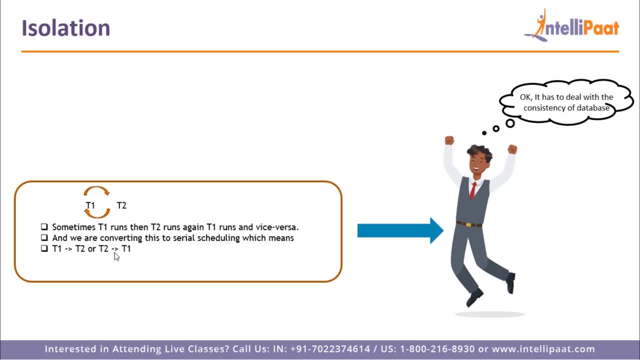 that is he understood. now i'll tell you the reason why we are doing serial scheduling, guys. well, we are doing serial scheduling because we want to achieve or maintain or attain the consistency in database. so i've already explained you what consistency means. that is the previous property, and we are trying to achieve that through isolation. okay, guys, a quick info if you want to. become a certified msg user, please subscribe to my channel and hit the bell icon so that you don't miss any of my videos. okay, guys, a quick info. if you want to become a certified msg user, please subscribe to my channel and hit the bell icon so that you don't miss any of my videos. 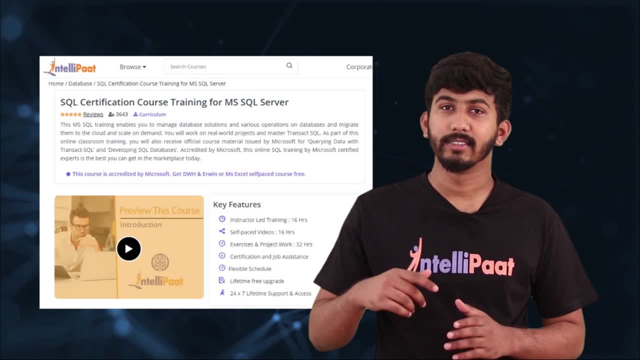 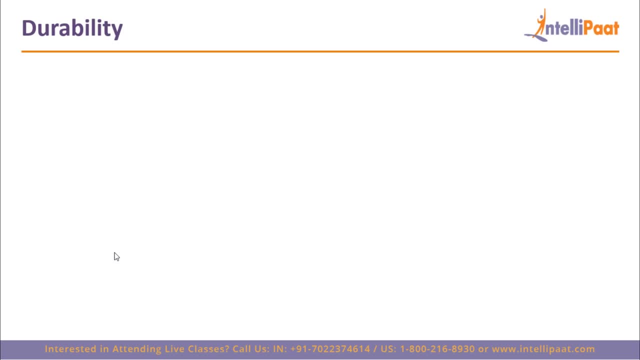 msql server professional by intellipaat. you can check the link in the description. now let us continue with this session. now i'll move on and talk about the last property, which is durability. so durability is nothing, but it basically talks about all the modifications and updates which i'm going to do, or which i have done to my database. let's say i have made use. 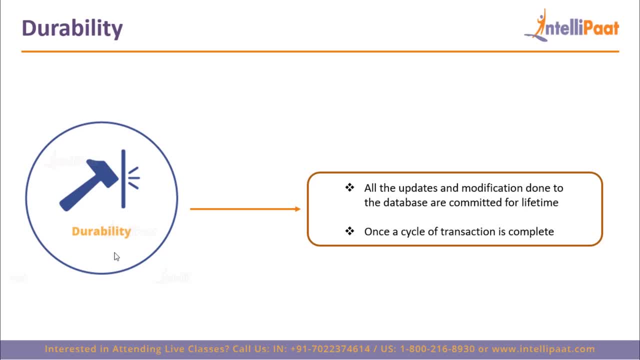 of a lot of sql query or statements like update, alter and you know things like that, or or or statements like that. then if i am writing commit that transaction or commit that db, then what's happening is that database will get committed for the lifetime, so that even when you there's 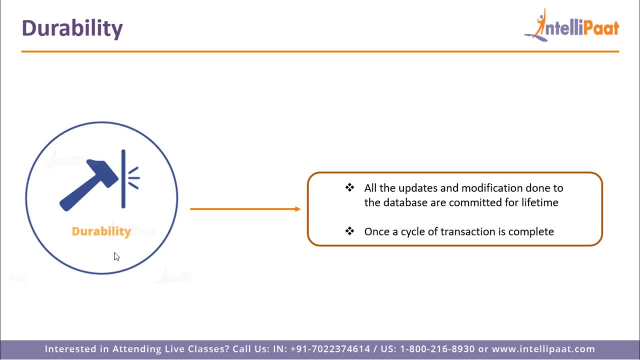 a power failure or your whole pc crashes. but when you format it or when you open your mysql or the sql server management studio and when you have that database existing, then you will find that database will be there and the changes, what you had done prior to that or previous to that, will be. 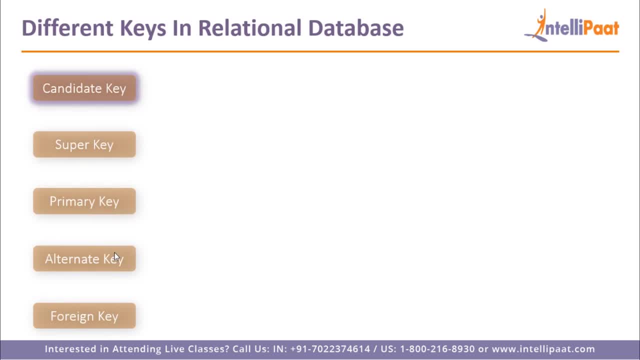 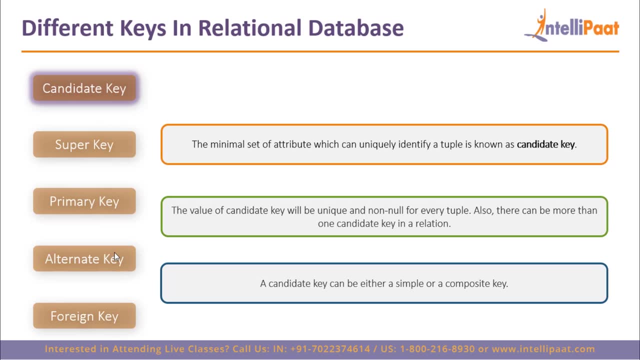 existing. now i'll move on and talk about the different keys which are existing in relational database. now, guys, this is very important from the normalization point of view, because when i get into that whole concept of normalization, you need to understand where i'm making use of the. 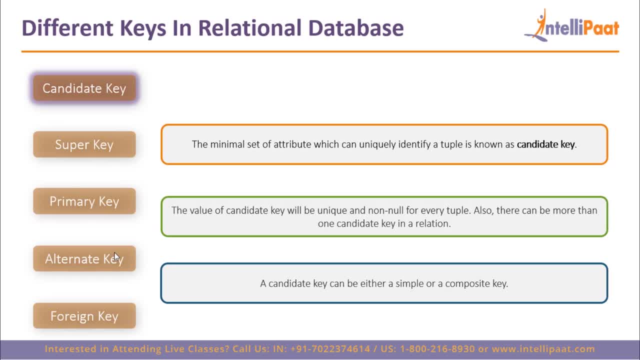 candidate key or where i'm making use of the super key, etc. so let me just start off by talking about what are candidate keys. well, candidate keys are basically the minimum set of attributes which can you uniquely identify all the records in a table. now, the value of candidate key will always be not null. 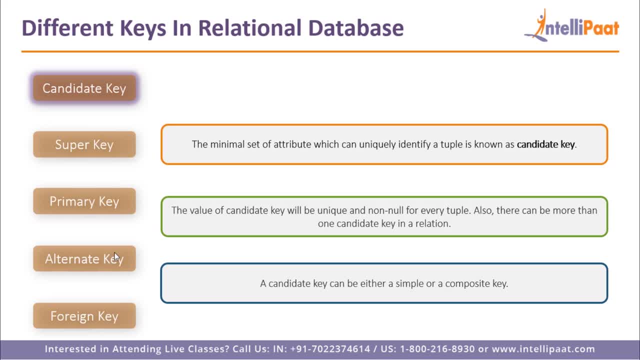 plus unique. you can think of candidate key as a primary key also, but in a relation or in a table there can be more than one candidate key. now, a candidate key can either be a simple one or there can be a composite key, that is, we have two keys which act as a candidate key. now i'll move on and 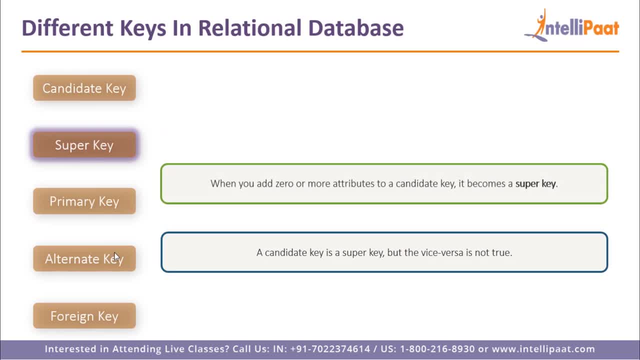 talk about the next key, which is super key. so the set of attributes which can uniquely identify a tuple or a record is known as a super key. so when you add zero or more attributes to the candidate key, it then becomes a super key and a candidate key is a super key. but a super key can never be a candidate key. 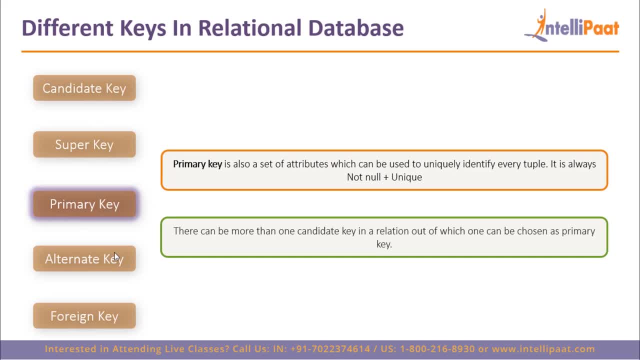 now i'll move on and talk about what is a primary key. well, a primary key is basically a set of attributes which can uniquely identify a table. now a can primary key basic essentially adheres to two condition, that is, when you have a table- let's say we have an employee table and it has different columns like employee. 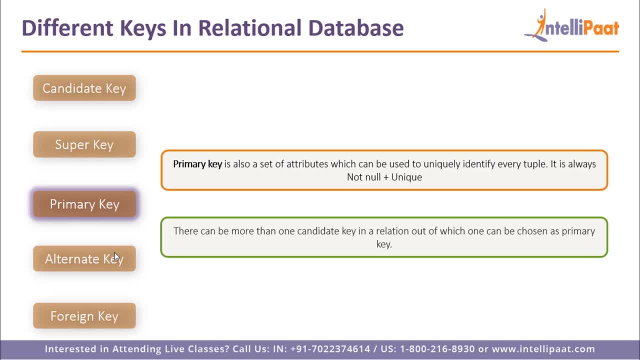 ID, employee name and employee age. so our employee ID will always be unique and that's how it becomes the primary key of that table. and the other part is it should never be null. so you cannot enter a null value into employee ID. if you do that, you will be violating the rules of employee ID of becoming a primary key. 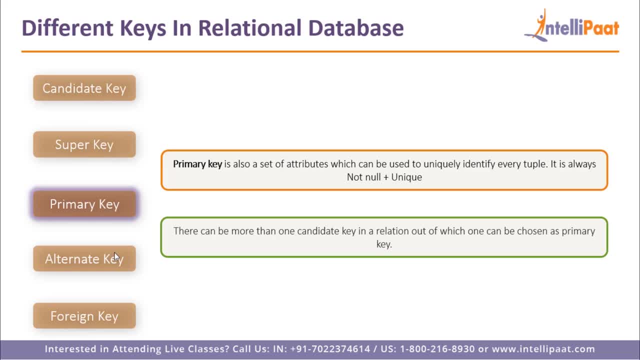 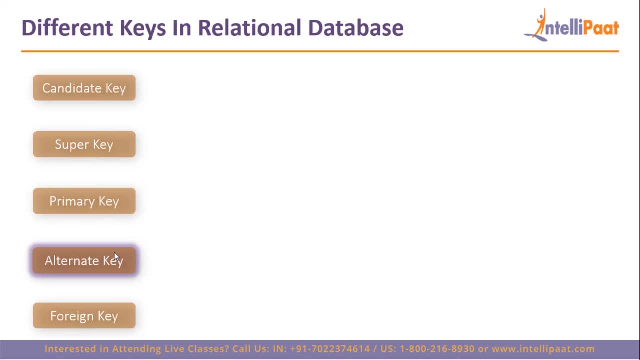 now, the second point merely states that they can be more than one candidate key in a relation, out of which one can be chosen as a primary. now let me talk about my next key, which is a simple key, that is alternate key. so any candidate key which is other than the primary key is called as an alternate key. but let me 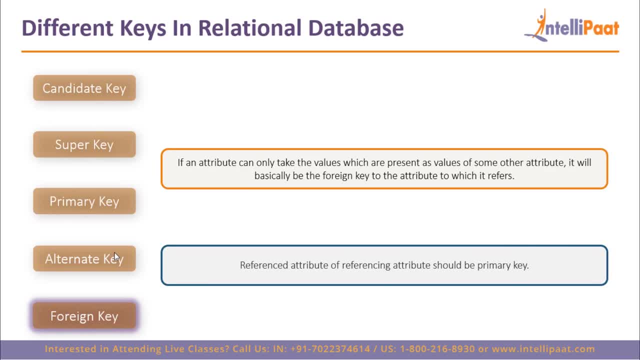 talk about my next key, which also happens to one of the most important keys apart from primary key. so that is known as a foreign key. so there is a for a very simple definition of a foreign key is what I can think of is: so let's say we have. 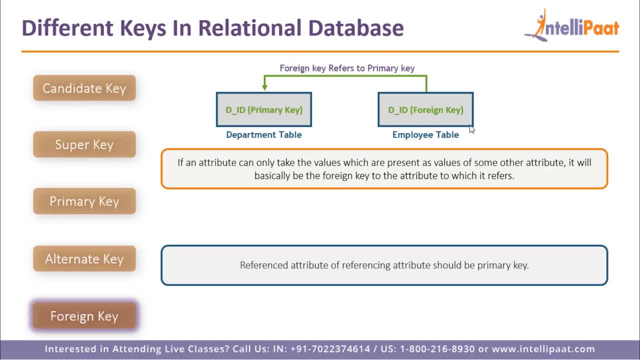 two tables, which is we have a department table and we have an employee table. so as you guys know that in department table we'll be having several columns which will be consisting of a department id, a department name, etc. now in the employee table we will again be having a department id. 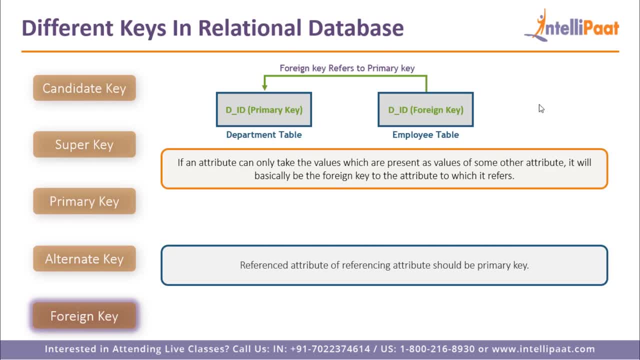 because that's how you can uniquely identify that employee. that okay, this employee works for this department. so let's say we have two departments, which are it and finance. now that will be acting as a primary key in the department table. now, when we go move ahead to the employee table, 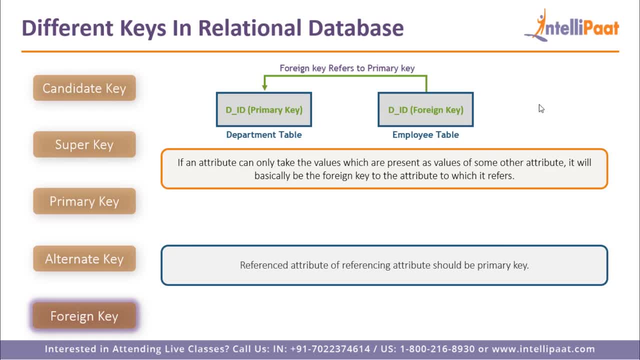 again, this department id will be acting as a foreign key. so a simple definition of foreign key- what I can think of is a foreign key- is basically takes into account attributes of the primary key of your parent table and that basically acts as the foreign key of your parent table. so let's say we have two departments, which are it and finance. now that 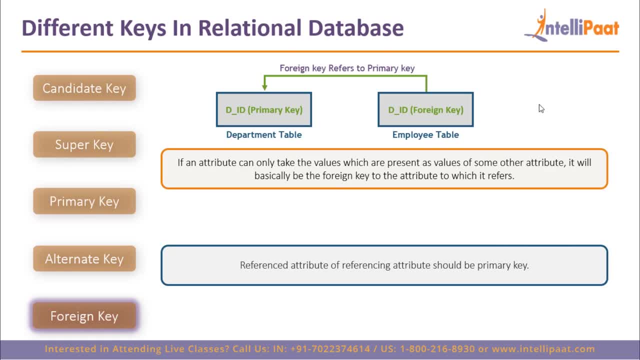 is, if you have an attribute which can only take the values which are present as values of some other attribute, it will basically be the foreign key to the attribute to which it refers. now the referenced attribute over here of referencing attribute should be primary key. so this is the 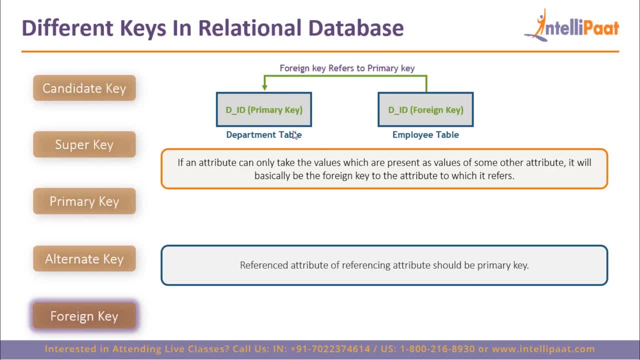 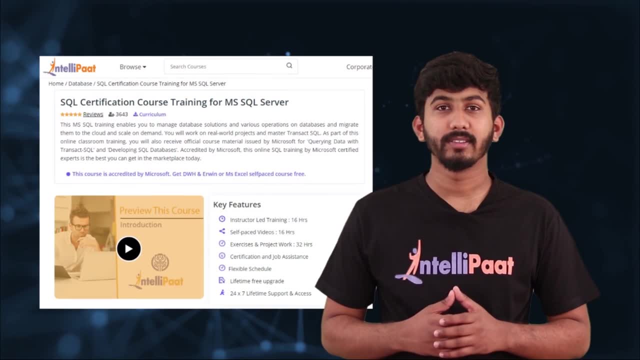 referenced attribute and then it is referencing to the di D primary key of the department table. okay guys, a quick info. if you want to become a certified MS SQL server professional by Intellipaat, you can check the link in the description. now let us continue with this session. 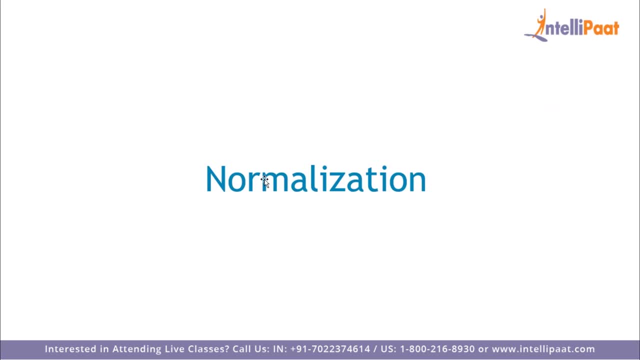 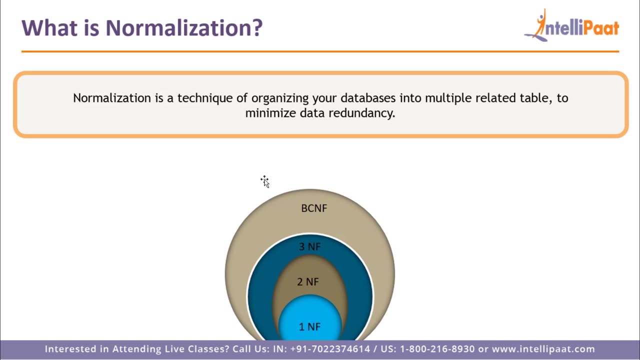 so let me just move ahead and talk about normalization. so the general definition of normalization says that it is a technique of organizing your databases into multiple related table so that you have to minimize data redundancy. now when I talk about data redundancy, guys, this term will always strike a chord with you, because data redundancy generally means that you are 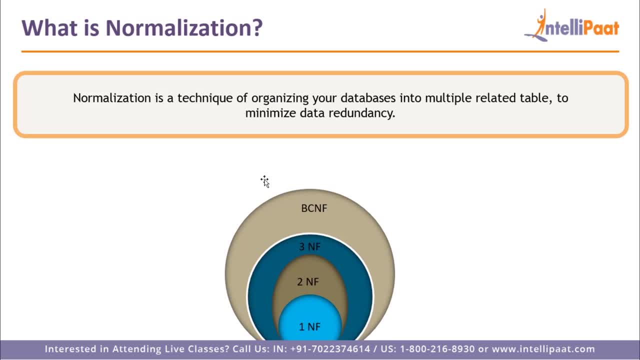 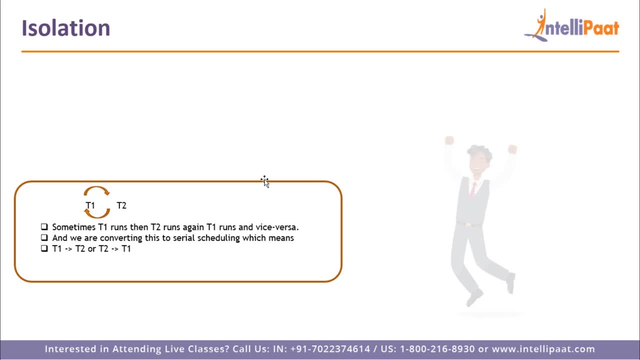 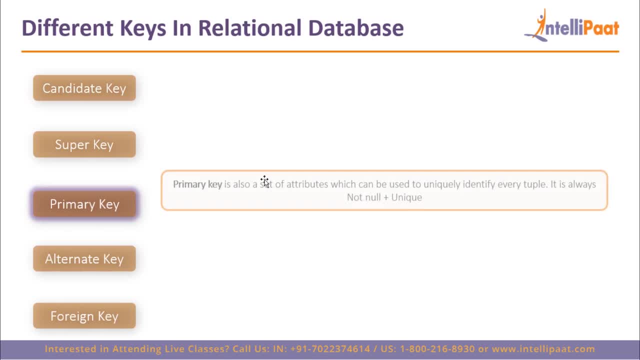 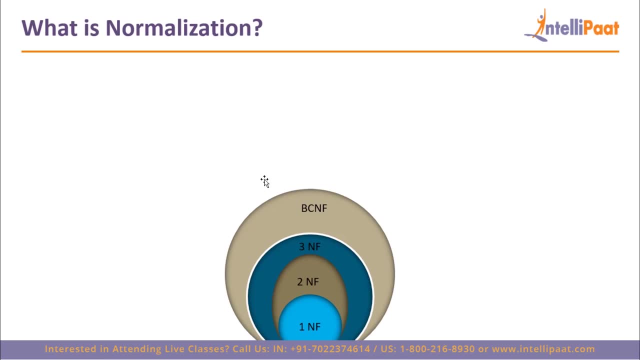 in my department table I have the D ID, I have the department name, I have other sorts of columns which are related to the department and in my employee table I have the employee ID and then I have the employee name- as a myth- and then I have the employee designation as: or the employee you. 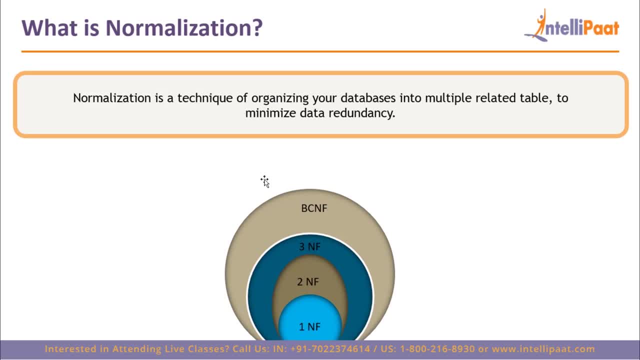 know, let's say, the department names. there are two names of department. so if there is IT department and finance department and that D name also gets carried in my employee table so that IT finance and you know that is getting repeated, so you multiple, you repeat IT finance, IT finance probably. 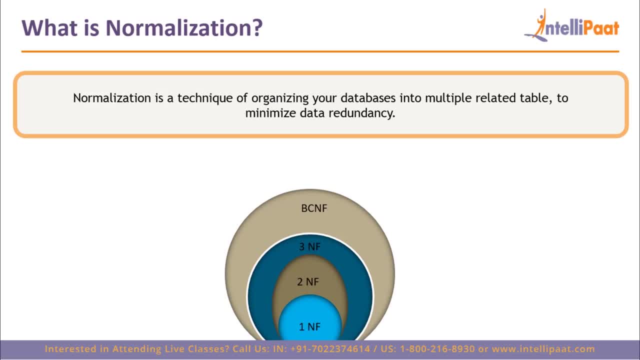 three, four times. so that can lead to data redundancy also, if I can think of a simple example. so let me take a student table. so under the student table I have HOD, I have branch, and the student ID is our primary key and the student names are different names, so let's say all of 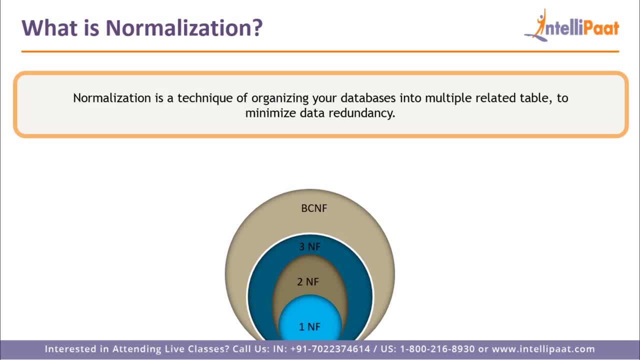 their branches are computer science, engineering, and their HODs are same, that is, Mr A. so what happens is this, Mr A, and computer science is a part of data redundancy, that is, the repetition of data is taking place. now, why is data redundancy is such a big evil for a DB? well, the reason is: 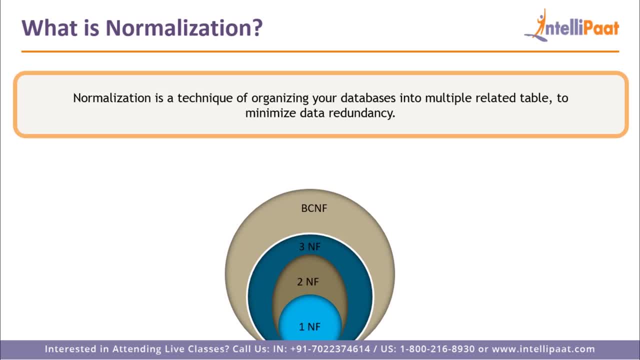 because it eats up unnecessarily extra space into the database, so that's why it's called data redundancy, the database which leads to different anomalies called as insertion, updation and deletion. now getting back to our topic of normalization, where normalization consists of four major parts, which are what? first, normal form, second normal form, third normal form and then the PCNF, that is, voice. 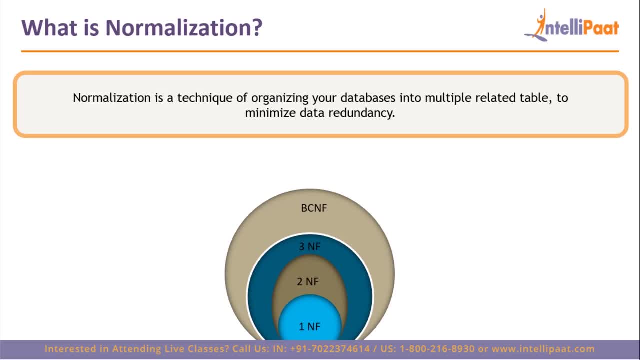 code normal form, also known as the three point five or higher normal form. well, if our database adheres to the first normal form, it need not go to the second normal form. or if it does not adhere to the first normal form, then it follows the higher normal form, that is second. 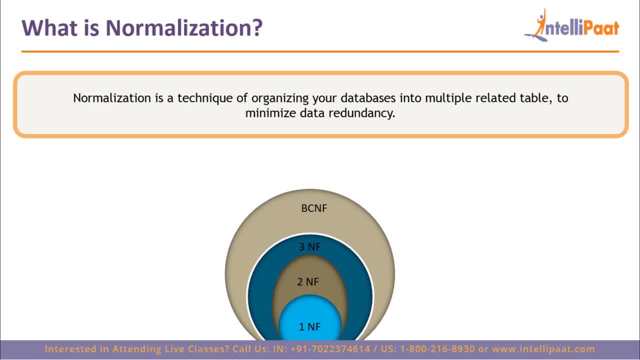 normal form approaches. even if it is not adhering to the second normal form, then it follows the third normal form approach, and if it does not follow B's third normal form, then it has to go through the BCNF form now. so these are the four major normal forms which are into existence or 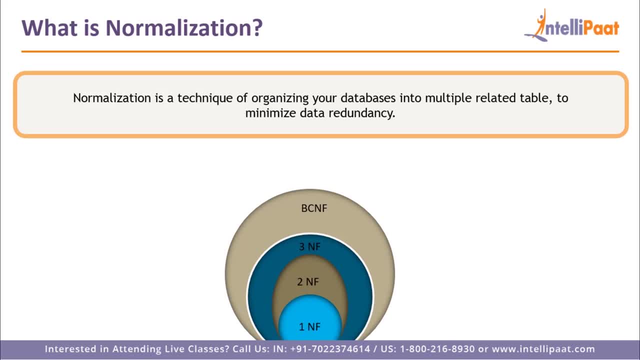 into picture. but the problem is, if the database, let's say it doesn't adhere to all these normal forms, then it has to again go through a fourth normal form, then a fifth normal form and the highest normal form, that is a sixth normal form. generally for database adheres to these four. 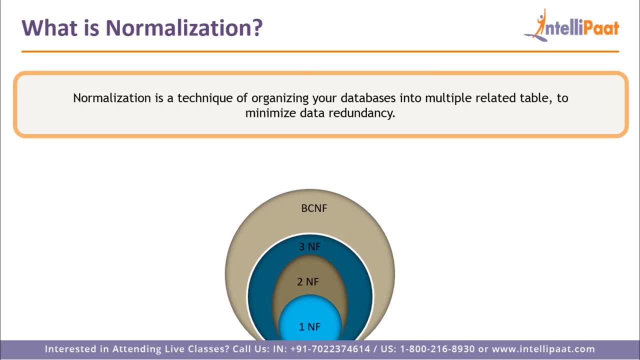 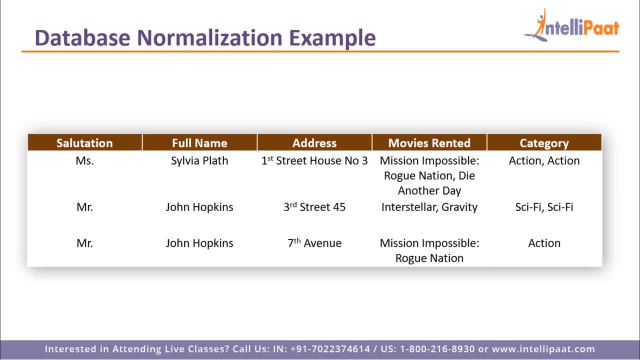 normal forms and it is called as a good DB. now moving on and diving deep to what are these normal forms? so, in order to explain that, what I've done is I have taken an example. so through this example, guys, this one single example, I'm going to be explaining you all the four normal 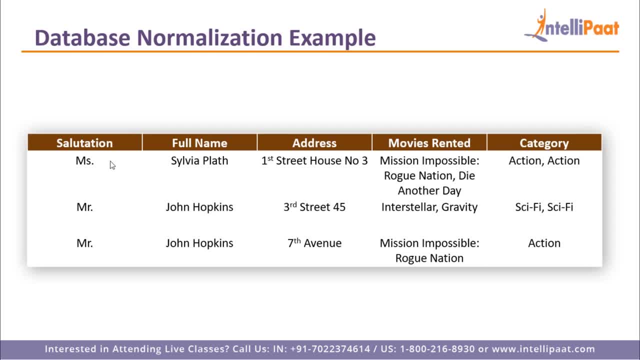 forms. so in this example I have taken a salutation as Miss, Mr and Mr and in the full name I have written Sylvia Plath and John Hopkins and John Hopkins. so the address of Sylvia Plath is first Street house number three, but the address of John 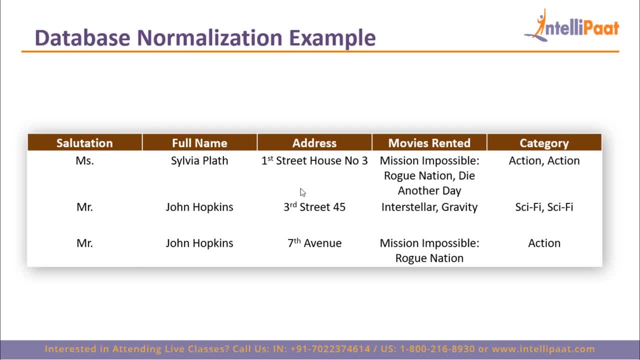 Hopkins is basically a composite attribute, as because I had explained you when I was explaining you composite keys, so it basically acts as a composite key of address where I'm just stating the third Street, that is a street name and the name of the house. similarly, in John Hopkins again, 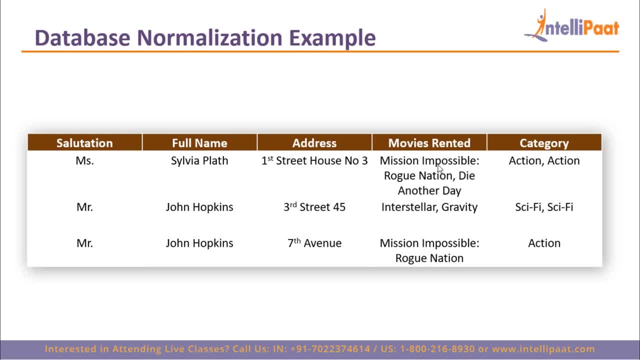 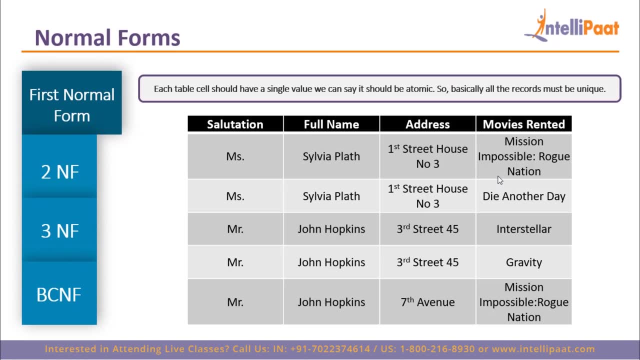 I'm stating the seventh Avenue, now the. these people have the movies rented, which are Mission Impossible, die another day, and the categories of it. now, when I talk, my first normal form, well, our first normal form states that it should follow the rule of atomicity, that is, each table cell should have a single value, or you. 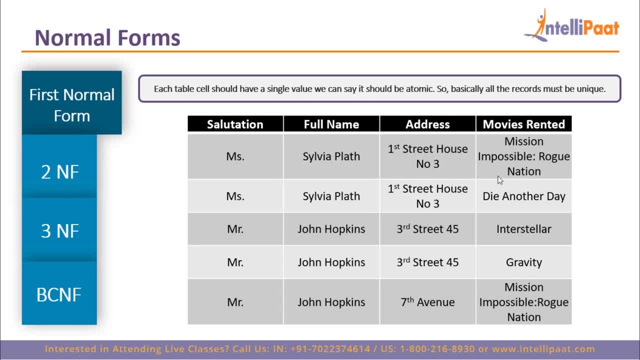 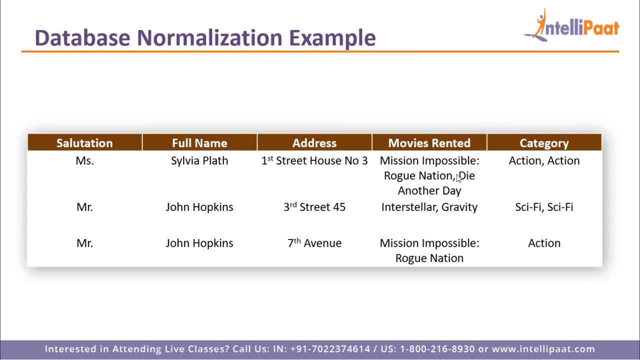 can say it should be atomic. so basically, all your records must be unique. so what I'm doing here is I have my salutation. that is my full name, Sylvia Plath. so Sylvia Plath, so previously, if you look at the previous table. so what happened? was this mission impossible, rogue nation and die another day were in the same row. 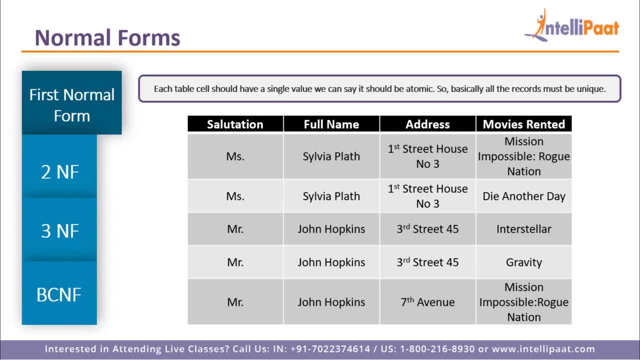 but now, when the table is in the first normal form, so these two get split into two different rows. so our name is again being repeated. similarly for John Hopkins, again interstellar and gravity is being, which was there in a single row, is now being divided into two different rows. but again, guys, this table has some. 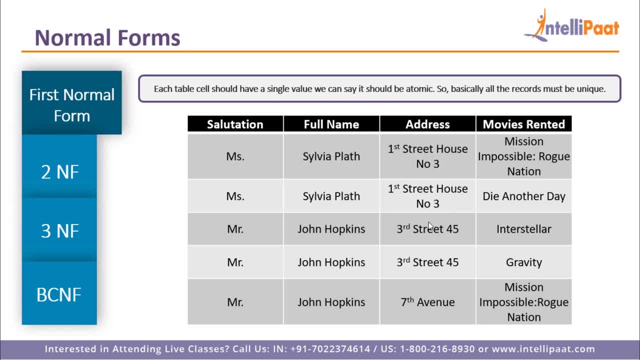 problem, that is, since I had already explained you that it consists of a composite attribute or composite keys, and then there's the full name John Hopkins. so this table is now being split into two different rows, so our name is. so now this table is again not fully correct, though it is adhering to the 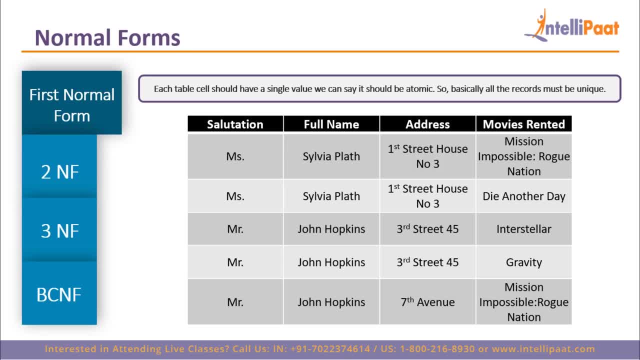 first normal form. what if we want to see the full address of the full name John Hopkins, or we want to see a single column primary key? so when I talk about that for part, I'll have to move on to my higher normal form. that is the second. 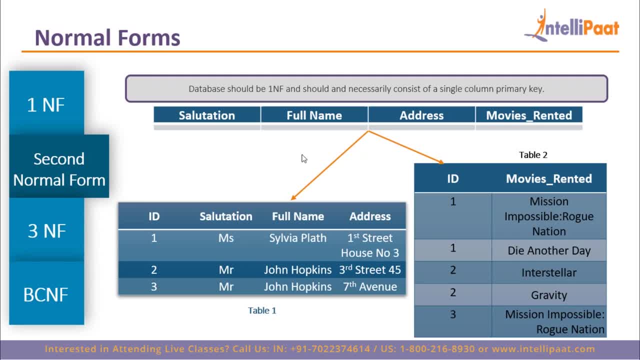 normal form. so my second normal form basically, or essentially, states that my database firstly should be in the first normal form and should be in the second normal form. and should be in the first normal form it should and necessarily consist of a single column, primary key. so now what I 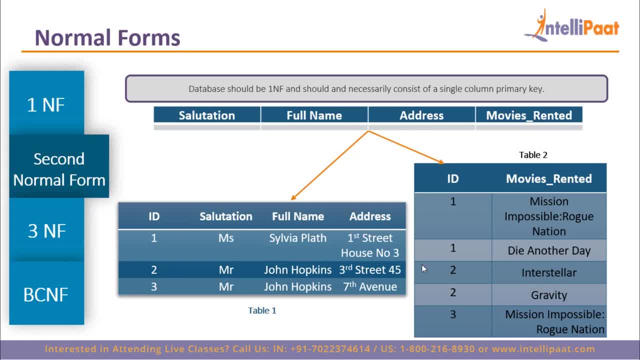 am doing is again, I have the same name, that is, John Hopkins, and I have the composite key attributes. but then here I have pretty much created a new table under which I'm adding a new ID, which is the primary key of table one, and this primary key of table one is now the foreign key of our table two. now I'll 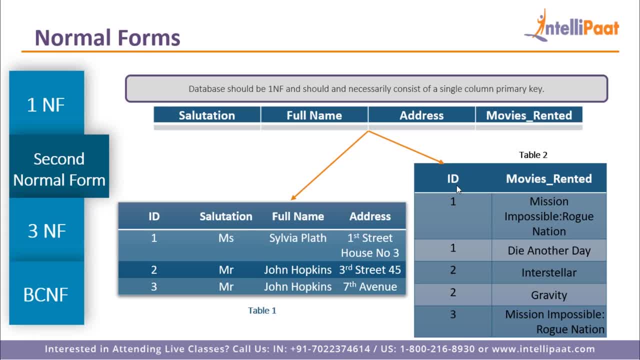 explain you how this is acting as a primary key of table one and how it is acting as a foreign key of our table two to. So let me just talk about the names. that is, Sylvia Plath has been given an ID of one Again. 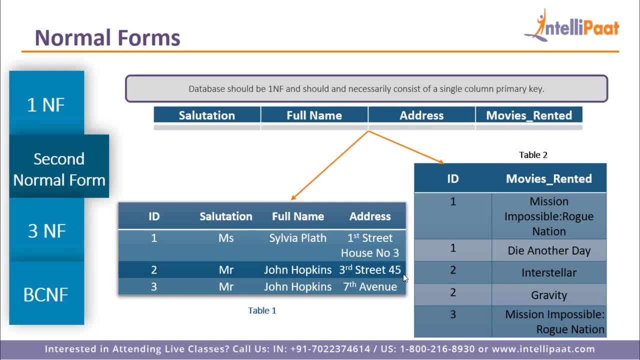 John Hopkins, who resides in the third street, 45th address, has been given an ID two, and John Hopkins, who resides in the seventh Avenue, has been given an ID three. So now, when I'm trying to differentiate on addresses based on our full name, I will be able to do that. That is leave. 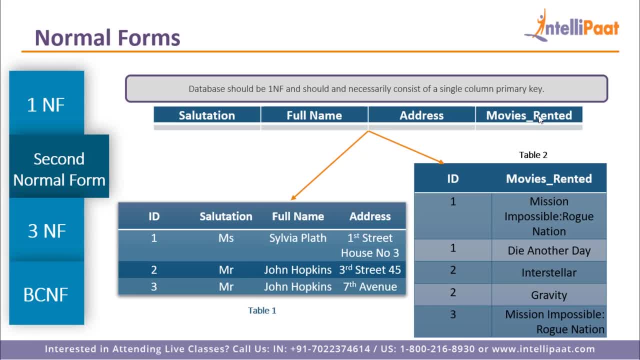 that aside, Now let's say I'm taking movies rented. So now our Sylvia Plath, who has been given an ID. one has rented the movie mission impossible, rogue nation. Again Sylvia Plath, who has been given an ID. one has rented another movie which is die another day. Now, John Hopkins. 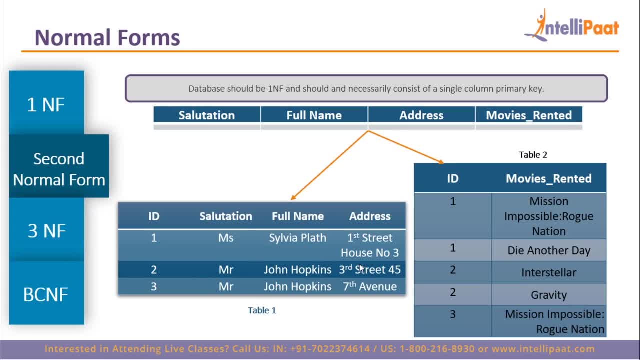 who has been given an ID two and who happens to reside under the address third street 45,, which is also the composite key, has rented a movie interstellar. And again, John Hopkins, with the ID two, who is Who's living in the address third street 45,, that is the composite key, has rented gravity. Now. 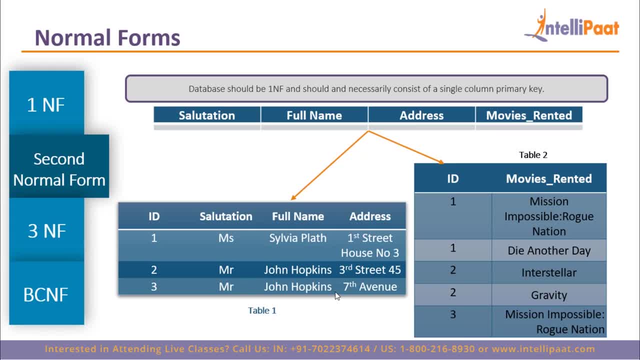 the third ID that has been assigned to the John Hopkins name again, but this time he's the person who lives in the seventh Avenue. So this is where the second normal form comes into picture, guys. So I have pretty much clubbed in a new column, that is, ID, which acts as a primary key of our table one. 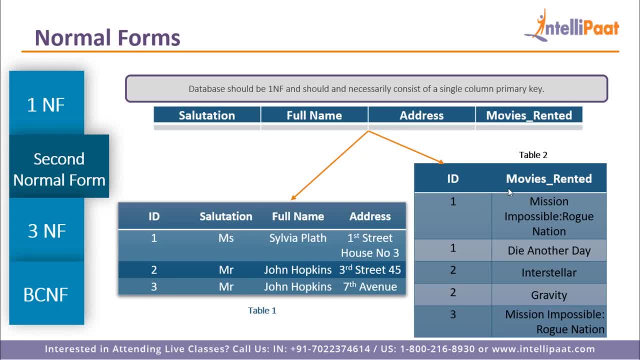 And this ID is then referencing to an article two as the foreign key, because this basically refers to the Parent primary key of, or the primary key of our parent table. And this is how we were able to solve the address issue, That is, the composite attribute issue, by simply providing unique values, or that's. 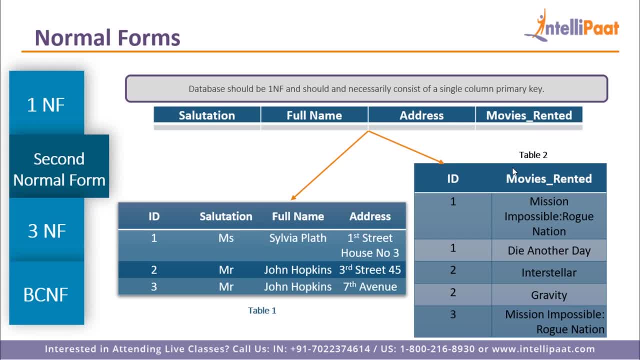 what our second normal form addresses on, That is, it should consist of a single column primary key, And that is what happening in our table one, And this primary key acts as a foreign key in our table. Now, guys, before moving on to third normal form, So what if I remove? 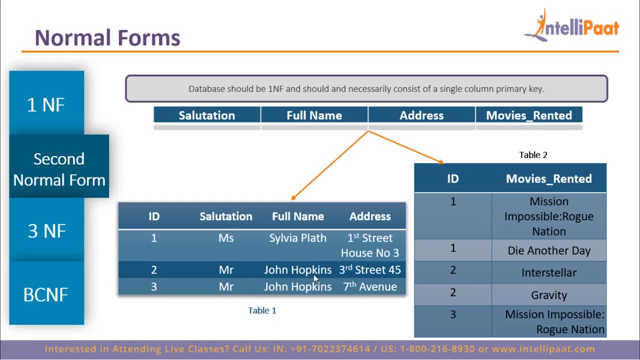 Full name, that is, John Hopkins. All right, So what if I remove John Hopkins, this name by, let's say, Alice Hopkins? So if I remove Alice Hopkins, then I'll have to change the salutation also, because Alice Hopkins will now be a Mrs And not a Mr. Of course the gender thing comes. 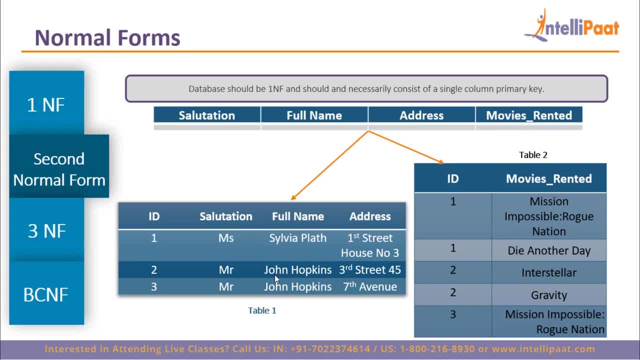 into picture over here guys. So if I take into account of Alice Hopkins, so what my point is? what I'm trying to explain is I'm basically trying to explain you a transitive function Dependency. So let me explain to you what a transitive function dependency means. So, as I 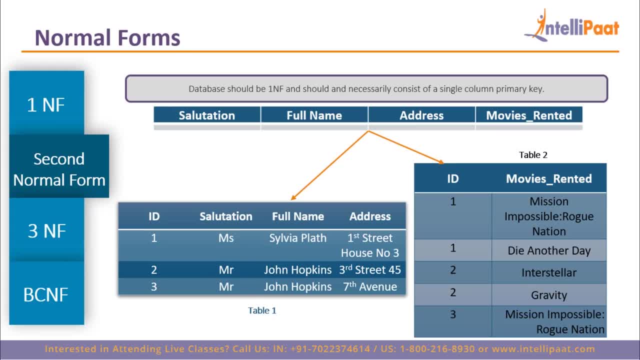 had already told you, if we remove John Hopkins and add pretty much Alice Hopkins over here, then I'll have to change the salutation also. So what it means is if you try to change a single non prime attribute or a single no key attribute and if the other non key attribute gets changed, 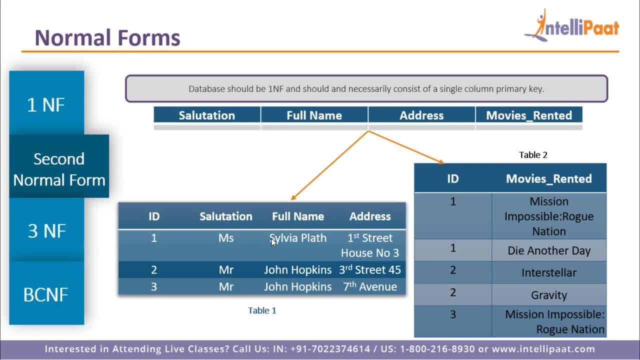 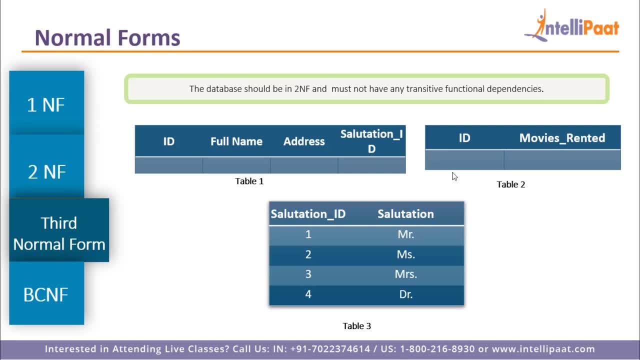 because your salutation is dependent on full name. then that part is called as a transitive functional dependency. So if you move on to a third normal form, that is, if you remove John Hopkins from the first normal form, I'll explain you why a third normal form basically talks about: 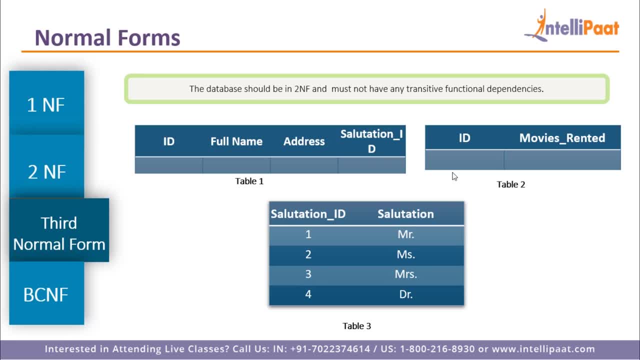 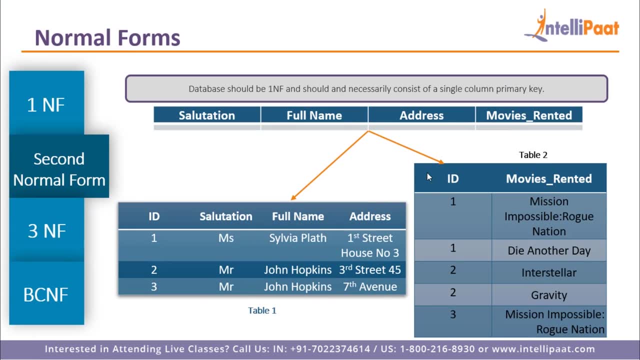 that the database should be in second normal form and it must not have any transitive functional dependencies. So when I move on to my previous table, so in this table, which is already in second normal form, guys, our salutation is dependent on full name. that is your non prime. 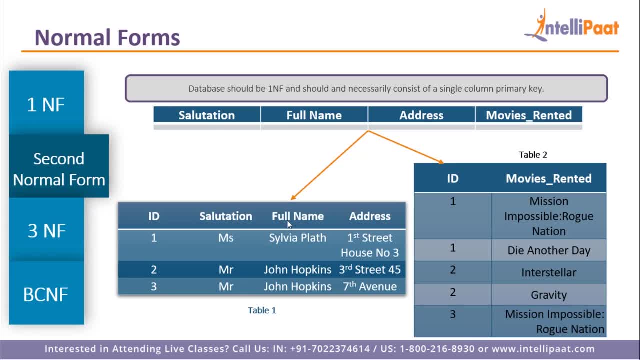 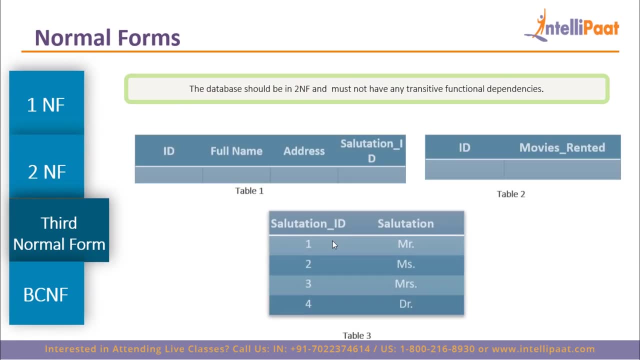 attribute should not be dependent on any other non prime attribute other than the prime attribute. So here our prime attribute, or the primary key, is the ID, But here there's a big blue pole, that our salutation is dependent on the non key attribute, which is full name. Now how do I solve this anomaly, Or how do I solve this ambiguity? So 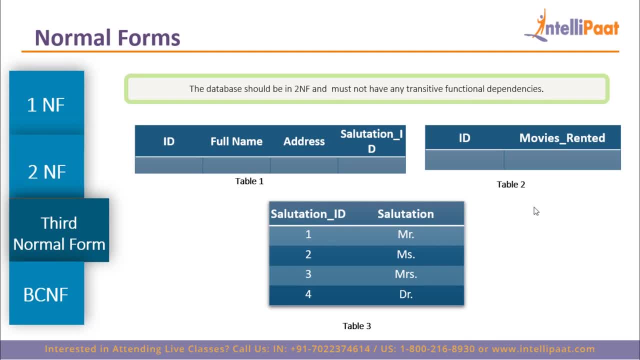 in order to solve this ambiguity, I had divided it into three tables. So, as you can see, guys, in my first table I have ID, which is the primary key, I have full name, I have the address, and then I have the salutation ID and my second table. So, again, our table one and table two is 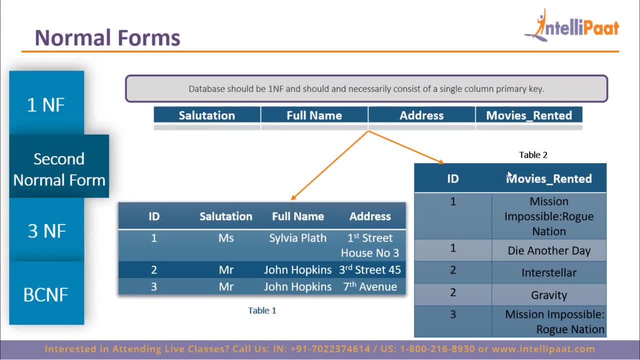 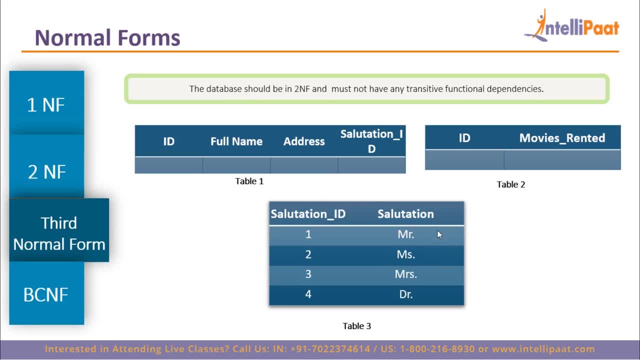 from the previous normal form, that is, it is the non prime attribute. So again, our table one and table two is in the second normal form. So it was. it's pretty much the same thing. Now the third table. what I have divided is here. I have divided the salutations. I have taken the salutation into. 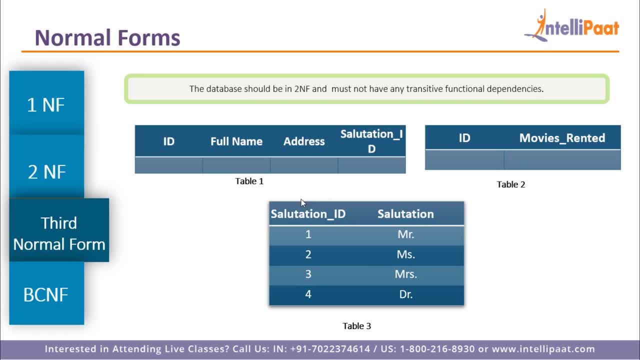 a different table And I have clubbed in a new column that is salutation ID. So now if I remove john hopkins with Alice Hopkins or john hopkins with you know how, about Hopkins, then I'll be able to write the salutation that will be the doctor or miss, and I'll also be able to provide. 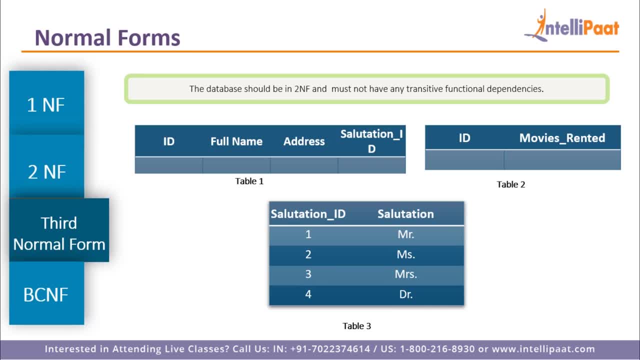 it With a unique key or the salutation or unique salutation ID. that is four and then can move up to five or six or seven. So this is what third normal form states, guys, that your database should be in two NF. So that is exactly our first and second table are in the second normal form. 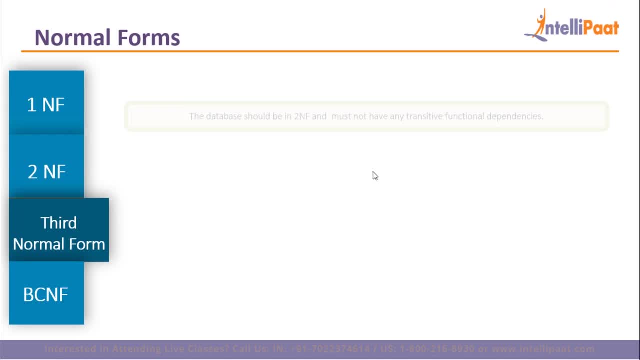 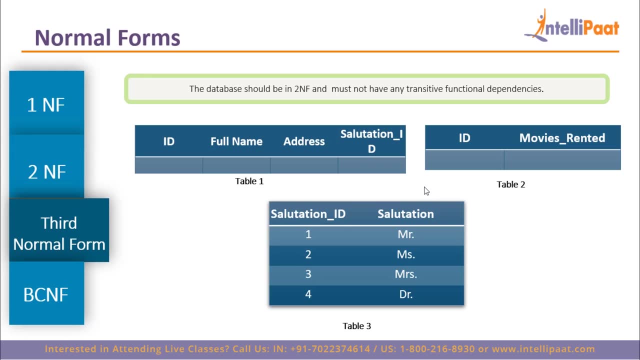 which I had shown in my previous example. And then if there are any transitive functional dependencies, that if one of the non key or the non prime attribute is dependent on the other non prime attribute, then that should not happen. And if such a case is happening, you take that whole. 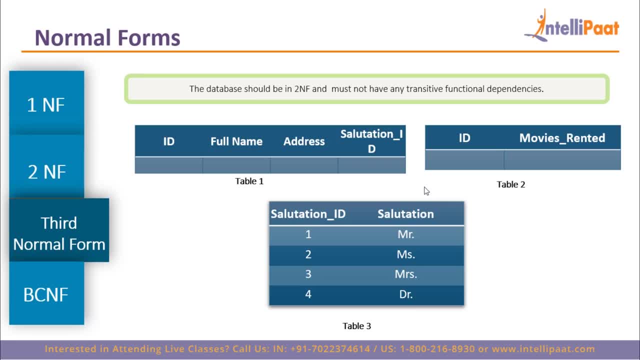 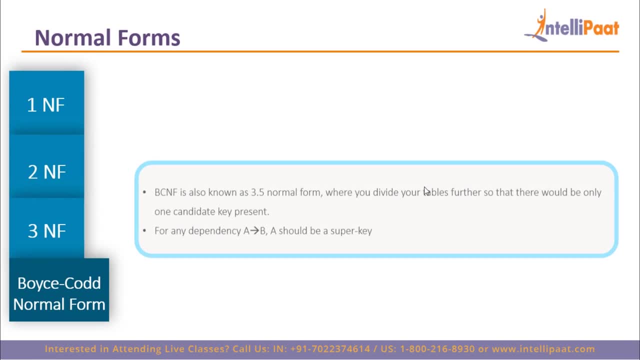 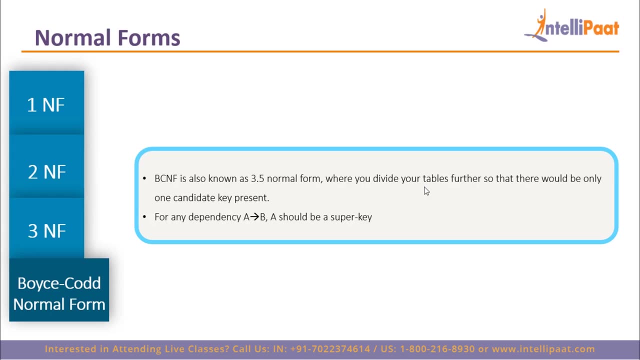 column out and make a new table out of it so that it is also dependent on the primary key. So this is pretty much it about our third normal form, Moving on to our last normal form, which is BCNF. So well, BCNF is also known as Boy Squad normal form or three point four non normal form. Here, 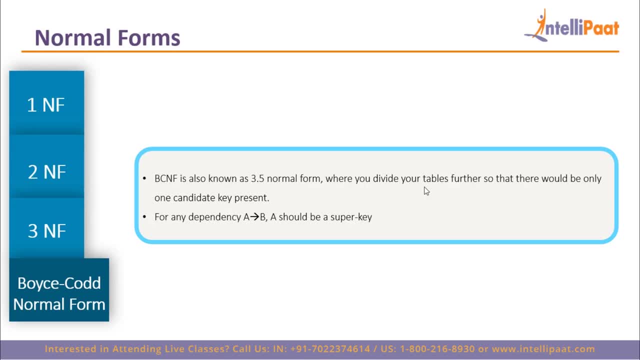 you basically divide your tables further so that there would be only one candidate key present. let me show you that by a small thing. So what if A is dependent on B here? so A should be a super key. Okay, guys, a quick info. If you want to become